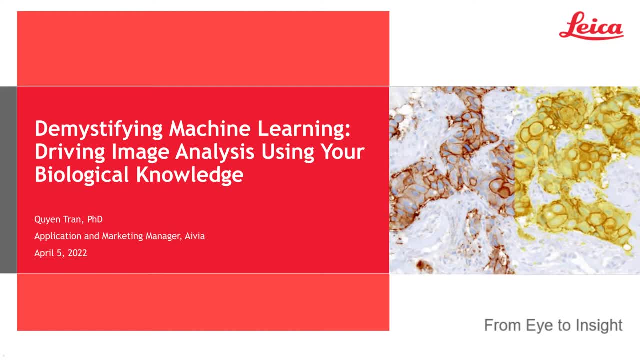 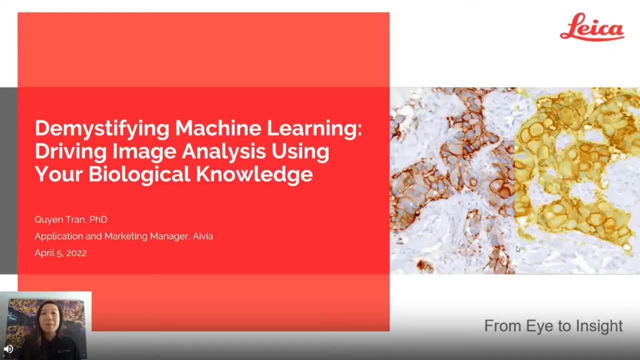 Microsystems. Dr Tran, you may now begin your presentation. Hello everybody, Welcome to this webinar and thank you very much for joining us here today. My name is Quinn Tran. I am the Application and Marketing Manager for the AVIA team here at Leica Microsystems. 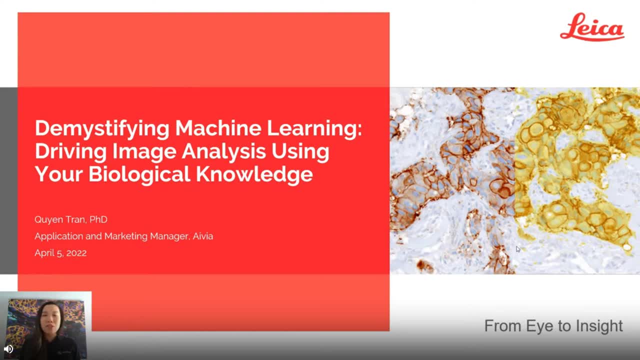 Today's webinar will be about demystifying machine learning, particularly how to use machine learning to drive your image analysis using your own biological knowledge. So let's quickly take a look at our agenda. First, I'll be talking to you about how to 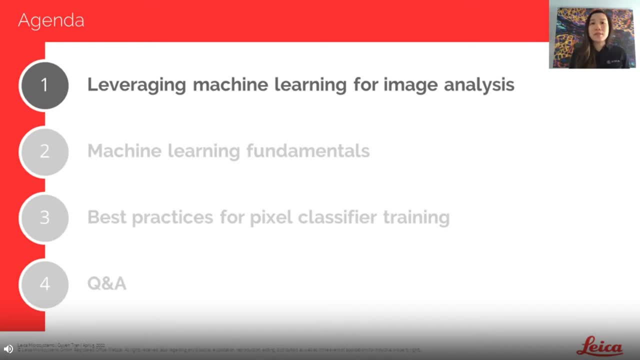 leverage machine learning for your image analysis. We'll then dive into some machine learning fundamentals, and then I'll share with you some of the things that we're going to be talking about today. First, I'll share with you some of my best practices for training. 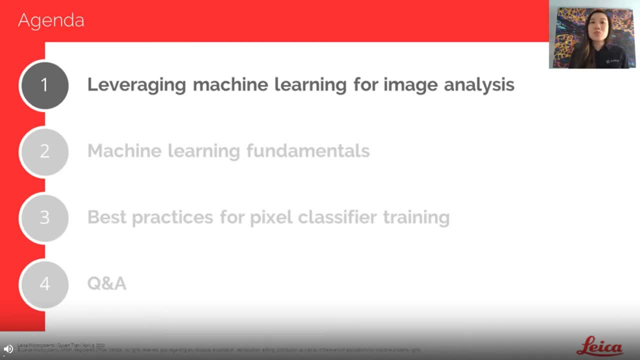 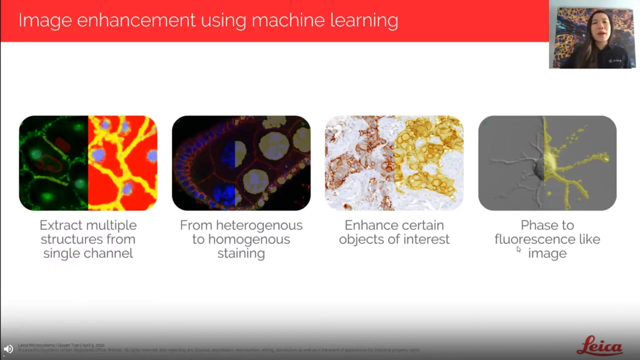 a pixel classifier, a machine learning tool that we commonly use in microscopy image analysis. We'll then end with a Q&A session, so that you have time to ask any questions you would like. So let's dive in. So I like to think about the ability to use machine learning. 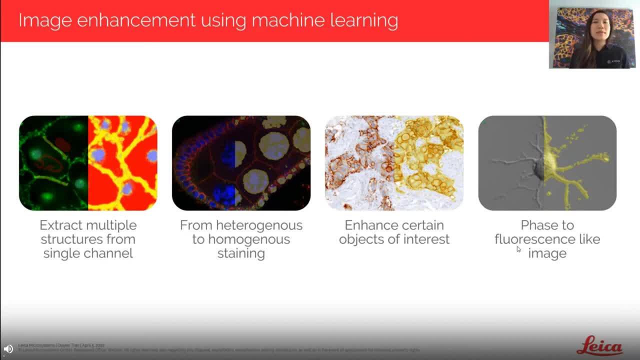 in kind of two broad categories. First is image enhancement for microscopy images. Now, I have four examples to showcase to you here, but I do want to mention this is not an exhaustive list of ways you can use machine learning for your images, It's just. 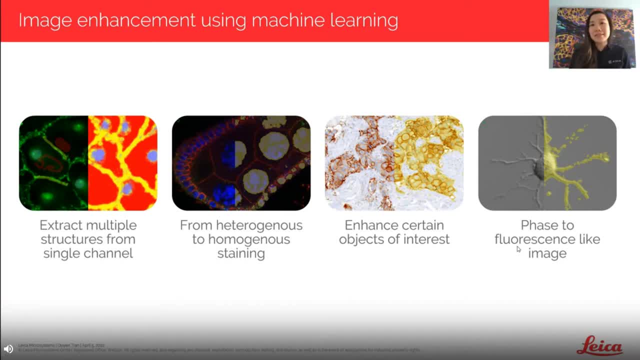 the four that I commonly see when I'm working with our customers. So the first example I have for you is this ability to extract multiple structures from a single channel. So here on the left-hand side in the original image, we have a stain that has stained the image. 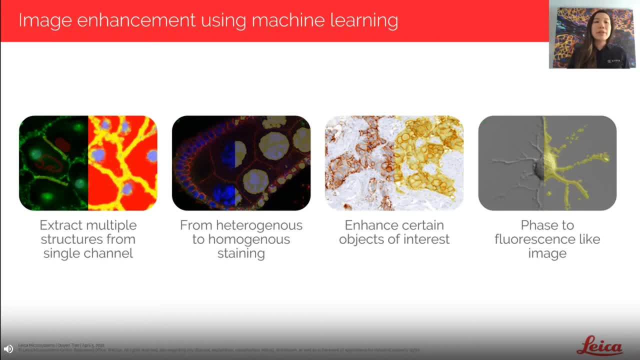 So we're going to take a look at how to do that. First I'm going to take a look at the cell membrane, the cell nucleus and also a bit of the cell cytoplasm, And for subsequent analysis, what we really want to do is separate these three components into three separate 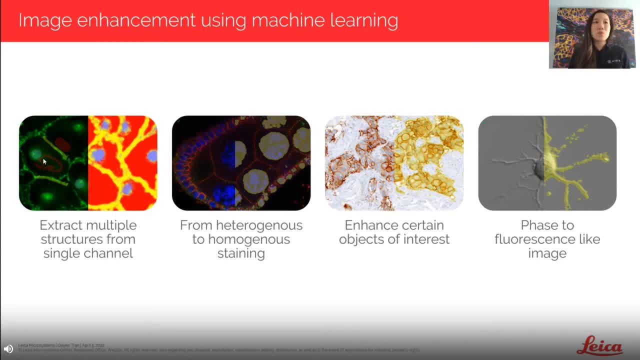 channels. So we have the ability to tweak and analyze and optimize the image analysis protocol for these three components separately. So, using the pixel classifier, the machine learning tool that we commonly use in microscopy images, we're going to take a look at how to do that. So the first example that I just briefly mentioned: we've essentially taught 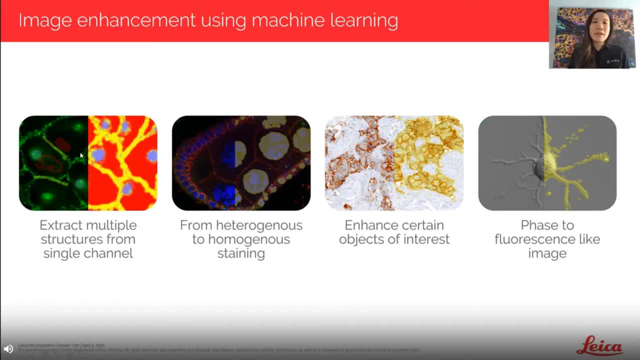 this software what each of these three components look like and then have separated them out. So now the cell membrane is in its own channel, depicted here in the yellow. The cell nucleus is its own channel, depicted here in the purple, and the same for the cell cytoplasm, depicted 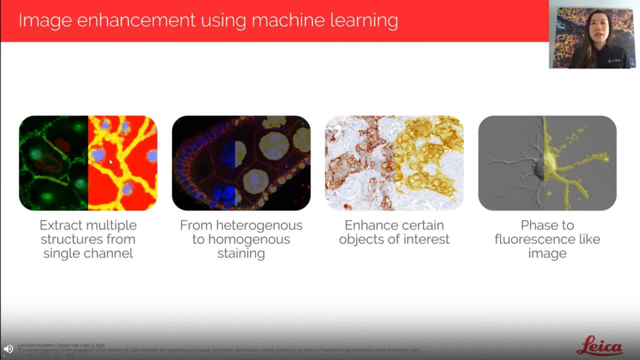 here in the red. So now when we do the analysis for these components, it's going to be much easier because they're separated from one another. My second example here is going from a heterogeneous staining to a more homogeneous staining And I think you can see that heterogeneous staining best than this nucleus, this large nucleus. 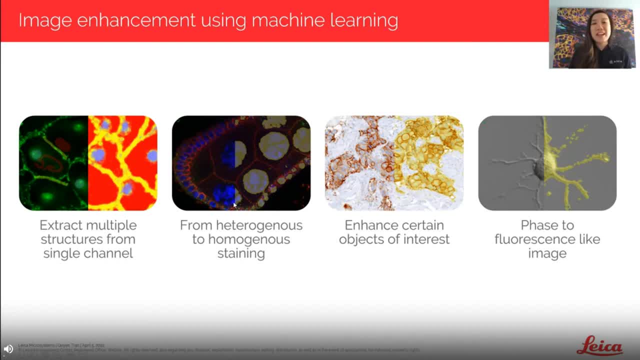 down here And basically because of the heterogeneity of this staining, it makes any image analysis- we do that our intensity base- very difficult. What's going to typically happen is that, instead of detecting this as one nucleus, it's going to break this apart into sorts of two different. 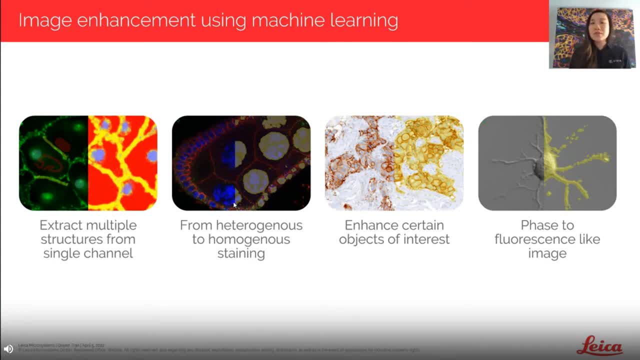 structures. I'm going to show you an example here of the heterogeneous staining. So if smaller pieces- which is not what we want to do, because that's not representative of the biological, the biological nucleus here- so, using again the pixel classifier, what we've done is essentially even out the staining. so now, 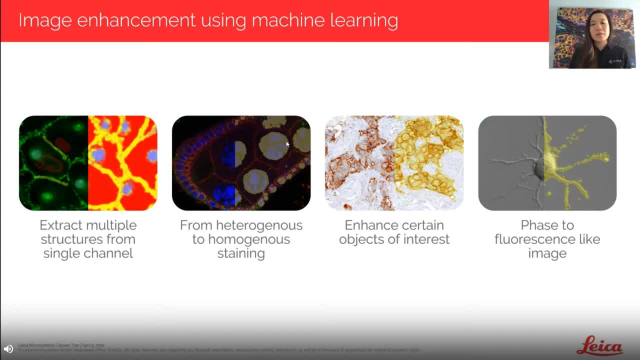 the entire large nucleus has a more consistent intensity level of the staining, so that when we do image analysis it's a lot easier to detect this as one whole piece. my third example is enhancing certain objects of interest in your images, and in this particular case I'm showing you a histology image. 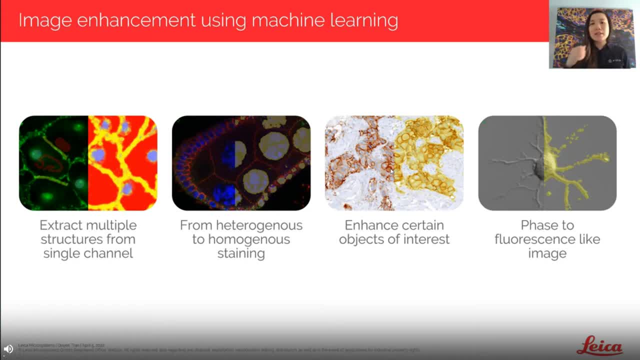 and what we wanted to pull out or enhance is these regions and these cells that have this stain. and again, using the pixel classifier, we've done that and that's depicted here in the yellow, so that we're really pulling this information out and away from the background of the rest of the image. and then my fourth example is going from a 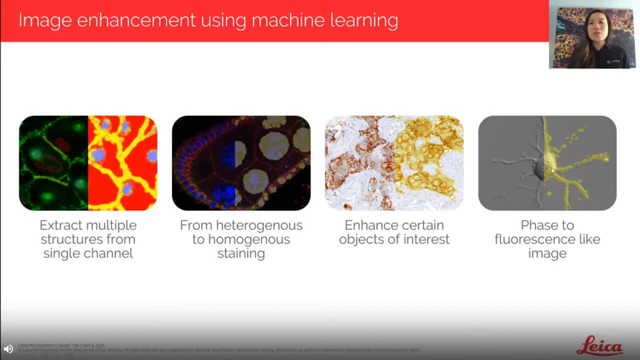 phase to a fluorescent like image. so here we taught the pixel classifier to detect this neuron, both the soma and the dendrites here that are protruding out, and it essentially creates a fluorescent like image of this neuron, which allows you to do any substance that you want to use in your image, and that's what we wanted to do. 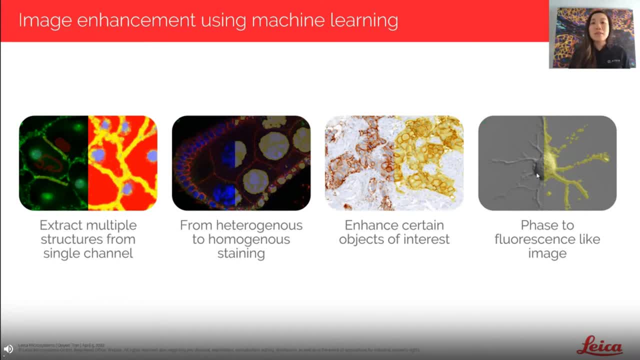 so that we're really pulling this information out and away from the background and you can see just enough detail of the transition that we've had made over the last couple of times, which I think is really important, because now you have an image that is really high, or has a really high signal or intensity of the 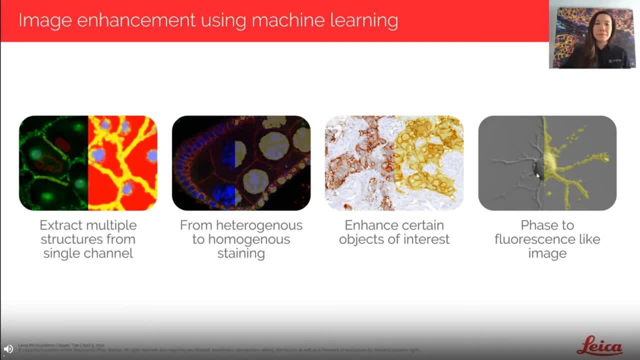 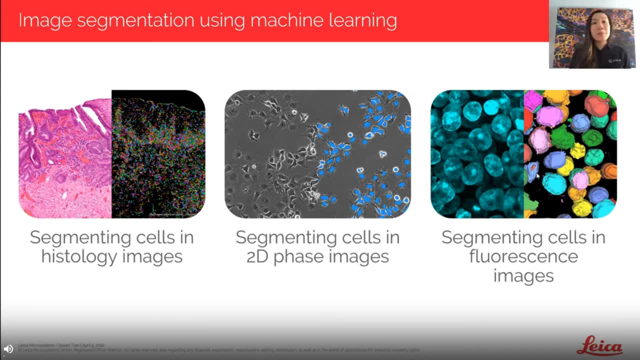 neuron versus a low signal for all of the other background components. now the other broad category I like to think about when it comes to machine learning and image analysis, it's the ability to go from the original image all the way. example for you here is segmenting cells in histology images. so this would allow. 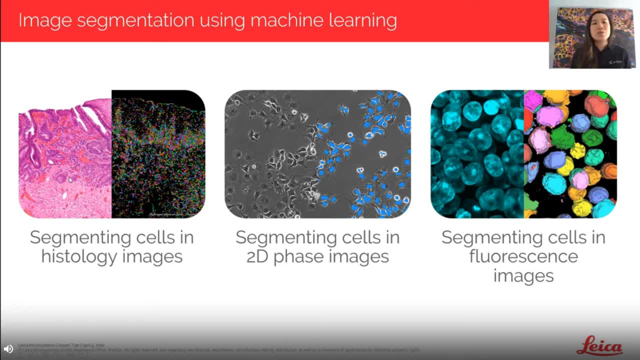 you to do cell counting. it would allow you to do cell counting in certain regions of interest. things like that are significantly easier to do now. the other example I have is segmenting cells in phase contrast image. so, unlike the example we talked about just briefly, where we enhance that neuron, we're now 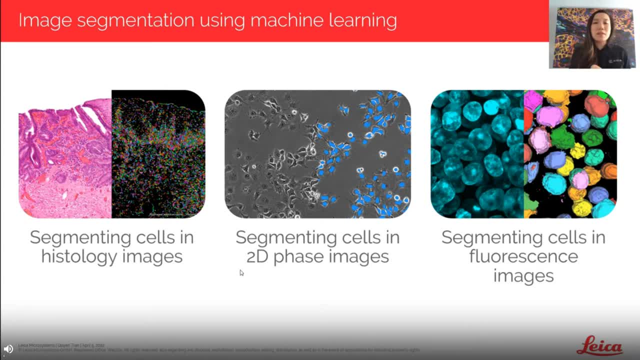 going from this- the phase contrast image- all the way to segmentation. this would make analysis, such as cell counting or understanding some confluency, a lot easier for you in these types of phase contrast images. my third example for you is segmenting cells in fluorescent images. so here we have the scenario. we 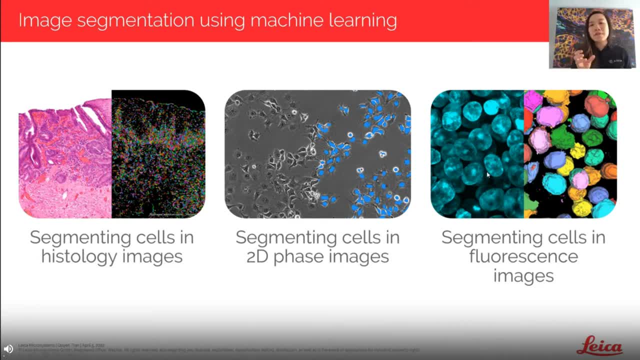 spoke about earlier, where the staining of the nucleus is heterogeneous, so makes that a little bit tricky to do using traditional intensity based threshold algorithms. so with the machine learning algorithm we're able to kind of pull all of this together and detect these nuclei in one large piece that is more. 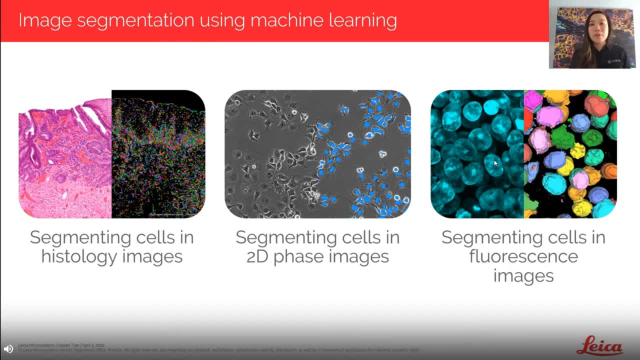 representation of their biology here. the other thing I would like to point out is when it comes to segmenting images- cells in fluorescent images. I also find the pixel classifier-classifier and to be really helpful in detecting cells that are of an irregular shape. they don't. 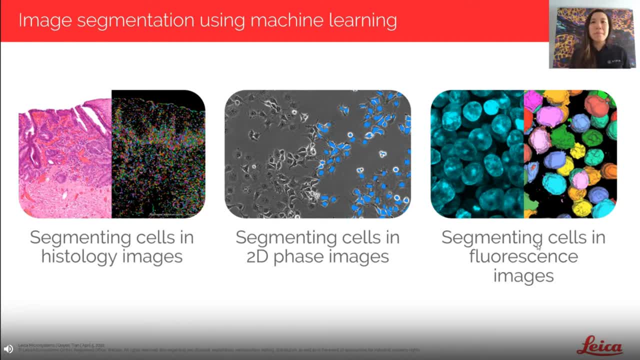 have this round globular shape which a lot of intensity based algorithms are optimized for because that's the most common way we see ourselves. but when we have something irregular, those algorithms may not work the best and I find that moving to a machine learning tool allows me to kind of be flexible and accommodate those irregular shapes, such as: 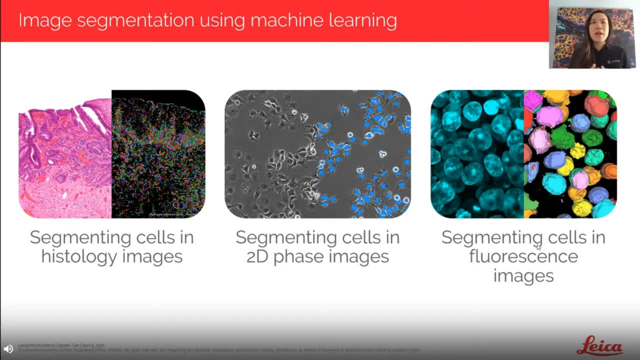 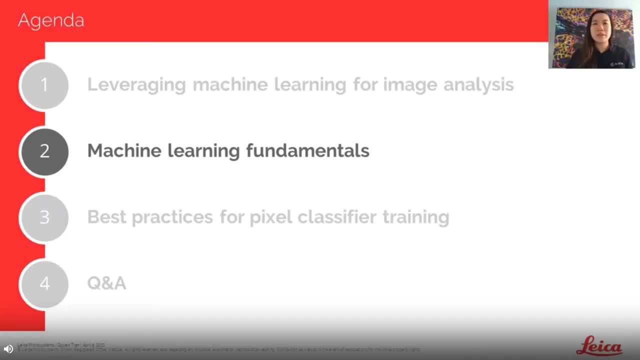 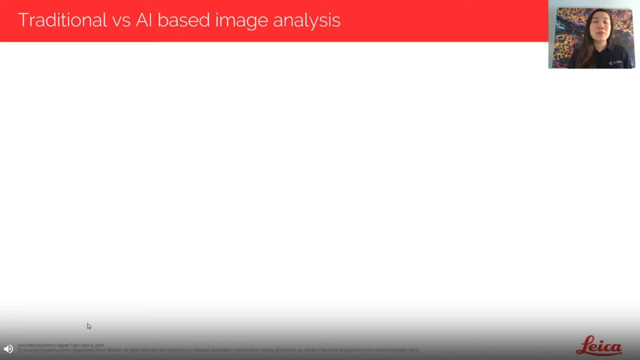 cells that are elongated or cells that have protrusions that you want to capture. All right. now let's talk about some machine learning fundamentals, And I typically like to start by looking at the traditional image analysis workflow and how that compares to an AI-based or machine learning image analysis workflow. 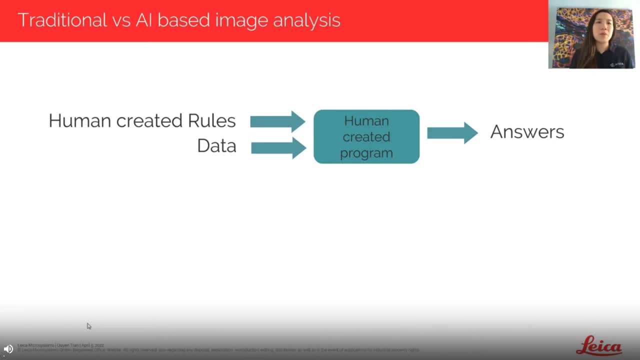 So in traditional image analysis workflow, we human beings, the expert, create the rules, Rules such as: my cells have to have an intensity level of 100 or above. My cells have to be in this particular size range. We take these rules and the images of the data and put it into the program. 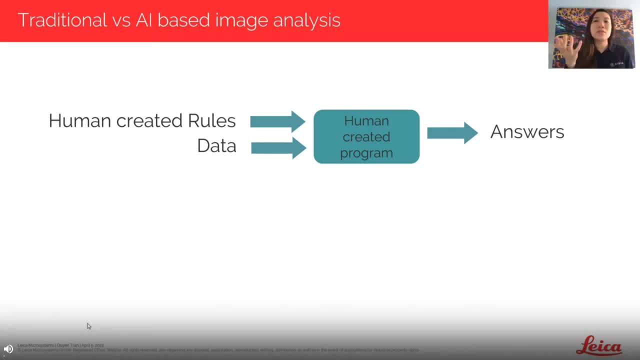 And the program provides us with answers. These are your detected cells For the machine learning framework. we're essentially flipping that script. What we're going to provide the framework is examples or answers of what the cells look like, what the objects of interest looks like. 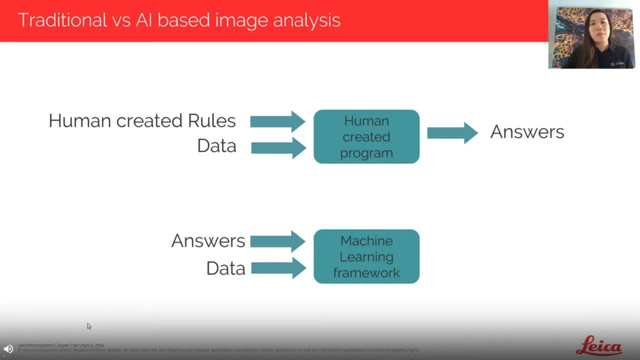 Feed the answers and the data into that framework And the framework provides us with those rules. So again, those rules that we just briefly mentioned: cell size, cell morphology, cell intensity profile. the framework gives us the rules that we need to make this cell or object of interest unique. 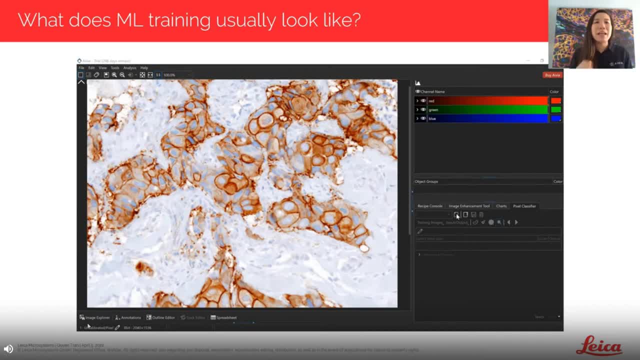 So, because of that flip, you might be asking: how does this actually work? What does it usually look like to train a machine learning algorithm? So this is a video showcasing you how the pixel classifier, a machine learning tool, in Avia gets trained. So in Avia, when we create a pixel classifier, we immediately get two classes. 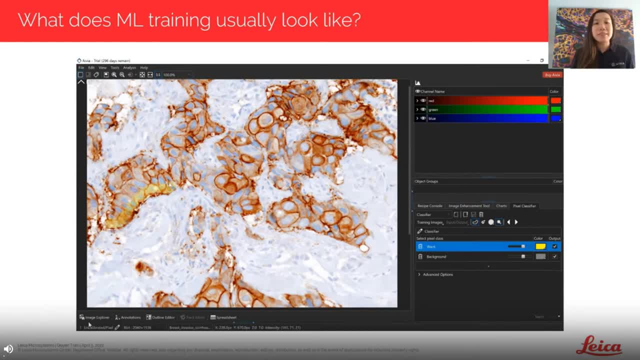 one with the background and then we provide examples, And this process is actually fairly simple because providing examples or answers is essentially painting pixels that make up what we want and then pixels that are considered background for us. So, again, that providing of the answer part is actually fairly simple and it's just a painting method. 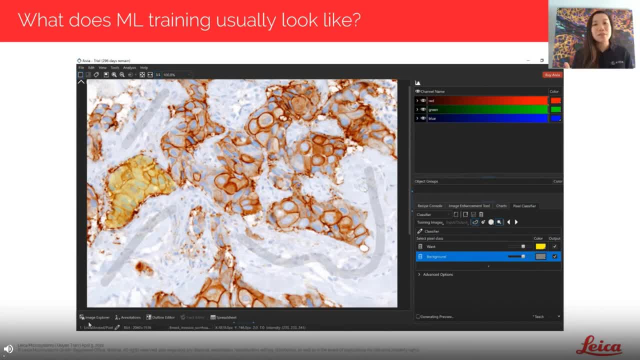 The answers and the data is now fed into the machine learning algorithm, which again spits out the rules, and then the rules are applied to this image. So, using that small subset of examples we provided, we create those rules and apply it to all of the pixels in the 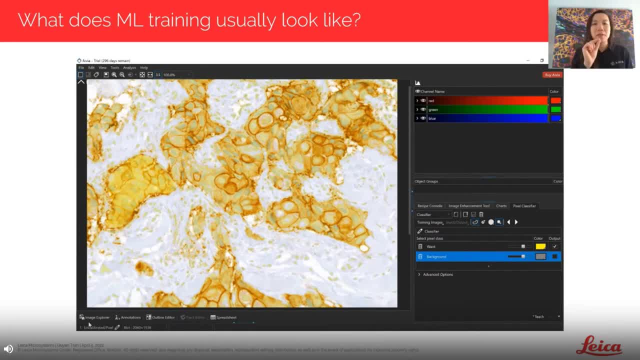 image and it enhances each of the pixels, It classifies each of those pixels as what we wanted in the yellow or background, kind of in this gray or non-existent color that we've shown here. So again, we're feeding the answers by painting those examples. 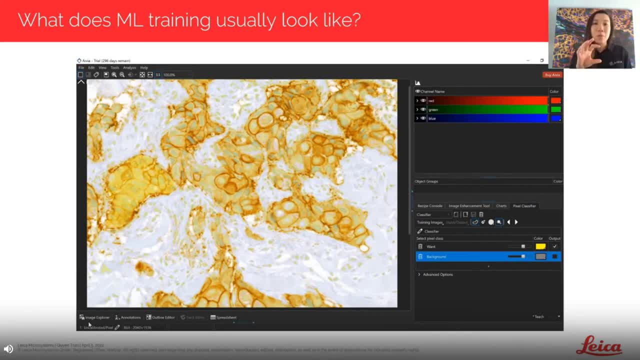 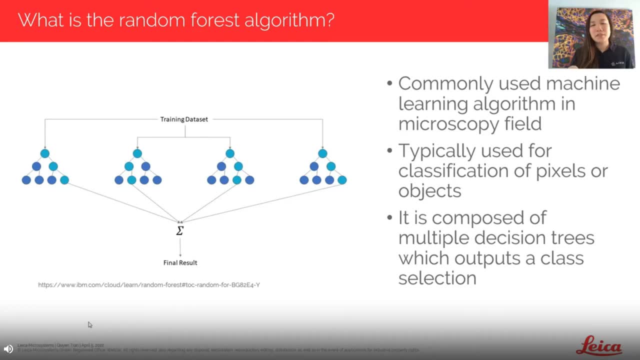 So again, it's a very simple process, but it's very easy and it's a lot of fun. So let's take one step further and ask ourselves and talk about the algorithm that is behind this tool, which is the random forest algorithm. It's a fairly commonly used machine learning algorithm. 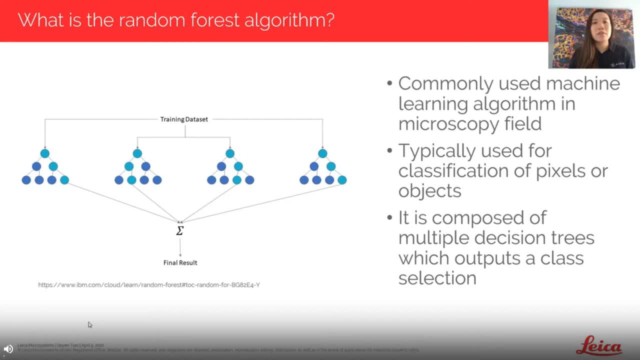 in the microscopy image analysis area And if you use other pixel classifiers before, it's probably the most common algorithm. So let's take a look at the algorithm. So the algorithm is basically running on the random forest algorithm and what it's typically. 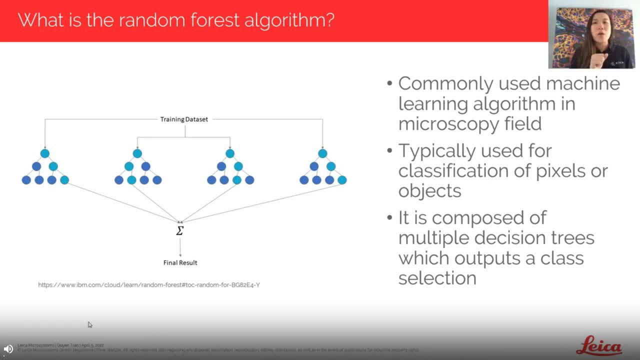 used for is the classification of pixels- what we just saw- or the classification of objects, So a classification of things, of cell A versus cell B, for example, And the framework here is shown on the left-hand side and essentially it's composed of multiple. 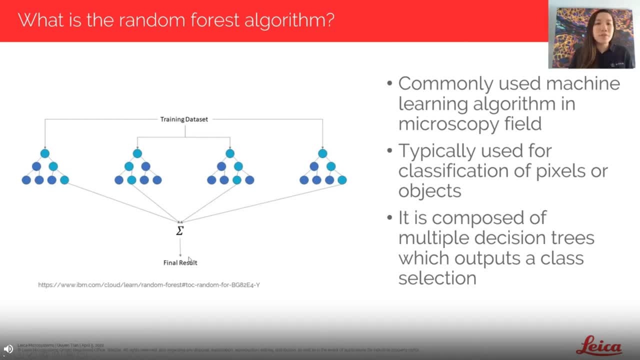 decision trees that collectively pool together to give you an output that selects a class. Is this pixel belonging to your what class? or does it belong to your background class? So that's really the output of the random forest algorithm. Now let's take a further step into this and ask: what's a decision tree? 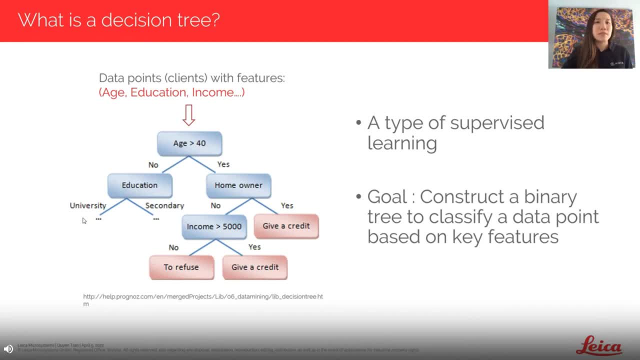 And it's essentially a type of supervised learning, meaning it requires an expert to help it with the learning process, And the whole goal of a decision tree is to make or pull together key features. that really allows us, allows it, to make the choice between what it is that you wanted or this is the background. 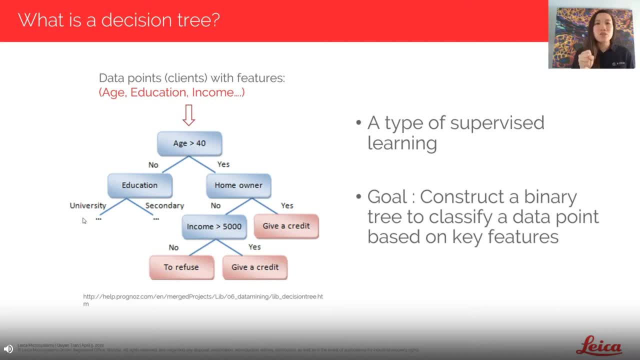 So again, these key characteristics and these features are pulled together in one decision tree to decide this binary choice. So my kind of non-microscopy example: here is somebody going in to get a loan and the loan officer you're working at, you're working with, might look at some key. 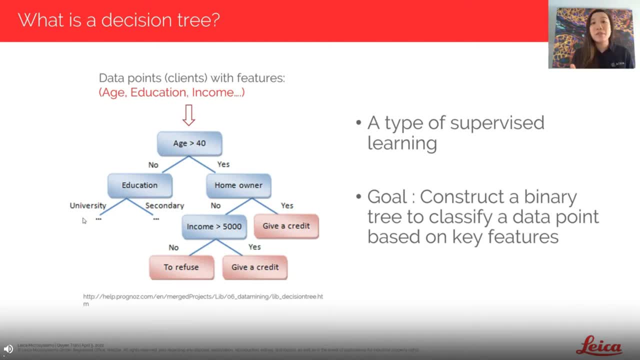 characteristics to decide whether to give you this loan or not. It could be your age, your education level, whether or not you've been a homeowner before your level of income, And these key characteristics, or these key features allows them to make this choice. 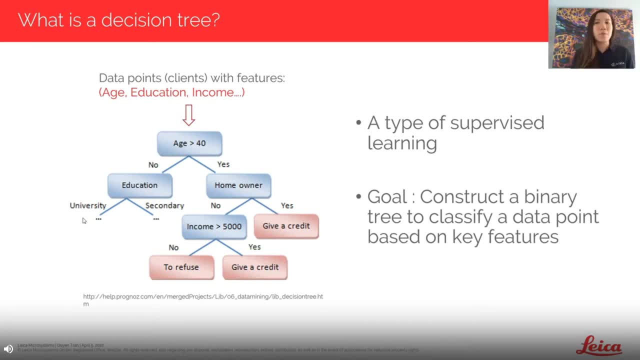 whether to refuse you the loan or to give you the loan. So we're kind of doing that in the same way that we're doing the non-microscopy data. We're trying to create a decision tree that pulls out the key features that make up your object of interest, to decide whether this particular 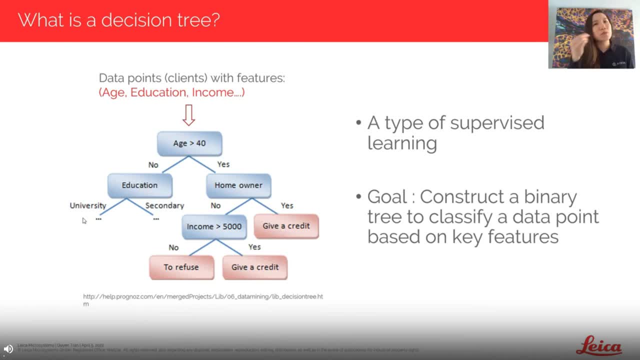 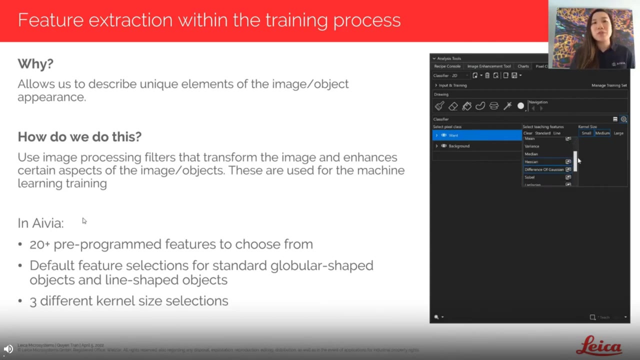 pixel or this particular object is what you wanted versus what is considered background. So I've said, feature a lot. What does this actually look like and what does this mean in microscopy images? So first of all, let's talk about why we do this. 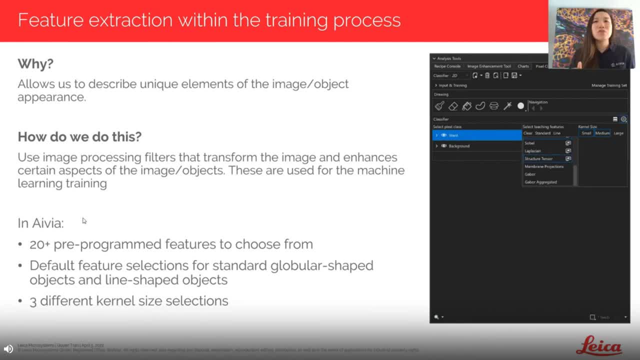 Essentially what it does is it allows us to describe the unique things, the unique characteristics of your object or your image, And this allows us to do it in a very systematic manner and one that pulls out these core features and these core components. So how does this actually happen? What do we do? And the process essentially takes: 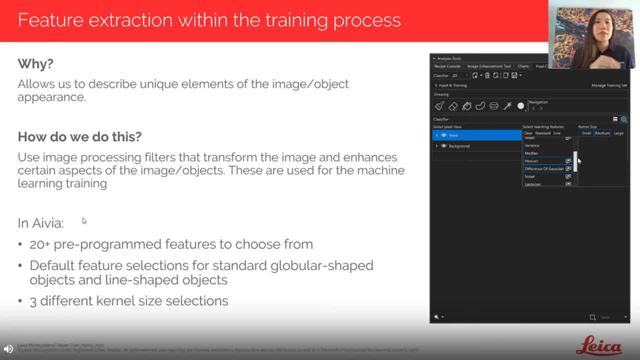 a number of image processing filters and applies it to your image, which transforms your image and enhance certain key aspects and certain key characteristics of the object that you're trying to detect in the object that you want. These transform images are then fed into the learning process to create the decision tree, to create the random force that we're looking at. 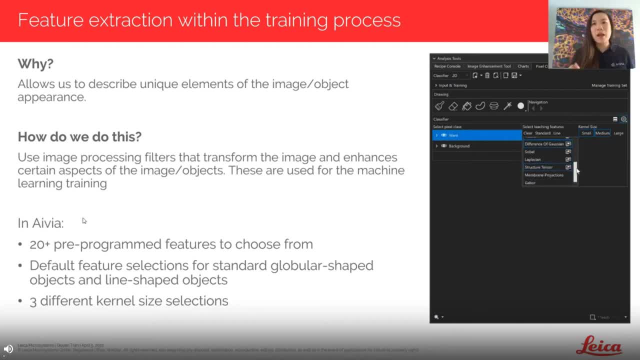 On the left, on the right hand side. here I'm showcasing the teaching features that are available in Avia. We have about 20 plus of them. We have also kind of organized them to into two categories for you, for anybody who's kind of starting out and don't really know. 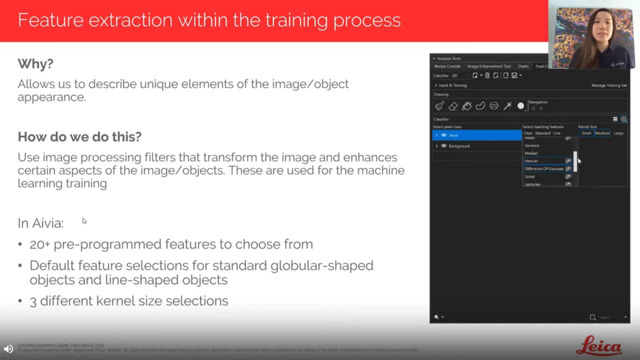 which features would be best. We've organized them into good features for standard globular round shaped objects or for line shaped objects. So you can always start there within Avia. You also might notice here that there's a kernel size selection. So in this teaching 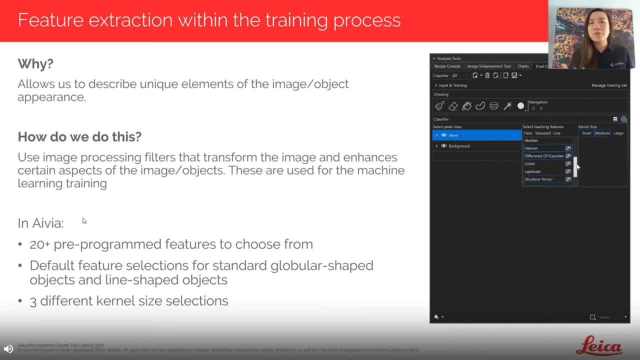 process. are your images or your objects of a smaller size of a larger size? things like that are possible to control in Avia too, And overall, the selection of teaching features and the kernel size is something that's typically available also in other pixel classifier. 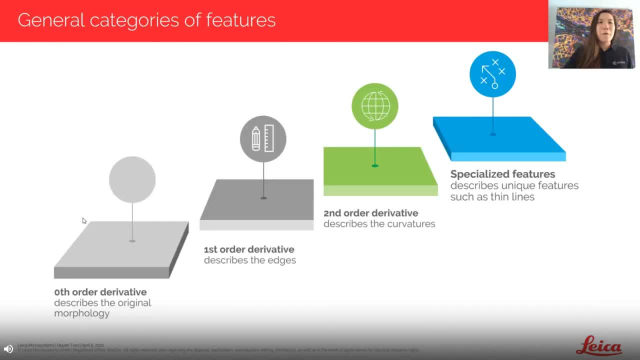 tools. Now, because there are 20 plus and sometimes even more of these features, I like to kind of think of them in general categories. It just gives me a good framework to think about which one may be critical to my objects and which one I might want to explore. 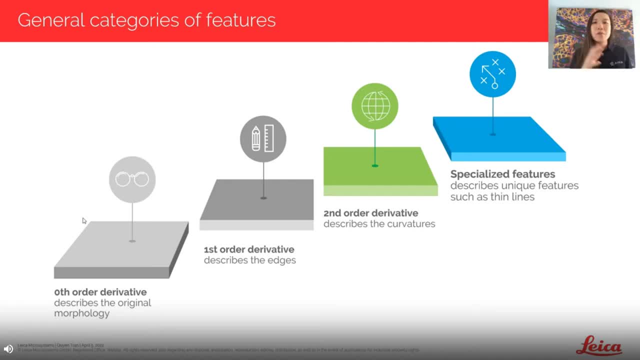 a little bit more. So the categories I think about here are zeroth order derivatives, which describes the original morphology of your image. We have first order derivatives, derivatives that's really good at describing edges of objects. second order derivatives, which is good at describing curvatures and, in general, most of the tools that they allow. there also have 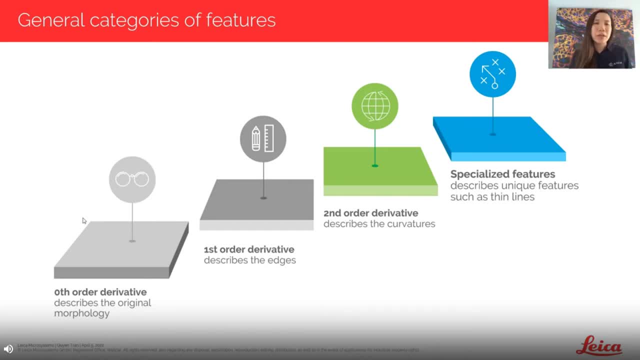 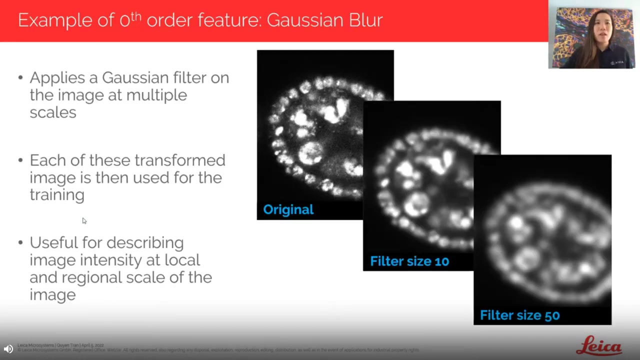 a set of what we consider a specialized feature that goes beyond the three categories we talked about. that describes other, more unique characteristics, such as really thin lines or something along those, those aspects. let's take a look at what an example what a zero order feature would look like. i've chosen here the gaussian blur for us to examine, and what happens here. 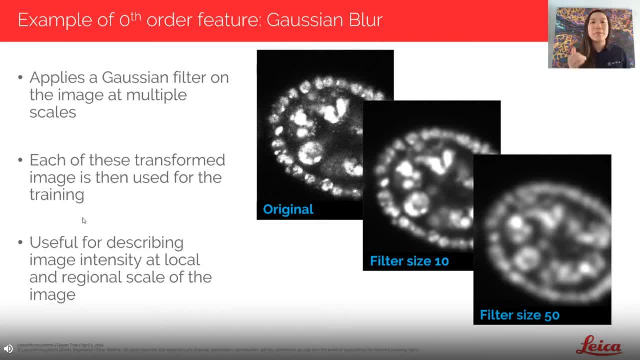 is, we applied a gaussian blur to the image at multiple scales. so, on the right, i've applied it at a scale of filter size of 10 and then a filter size of 50.. again, these transform images get fed into the training process, and what it's really good at doing is describing the 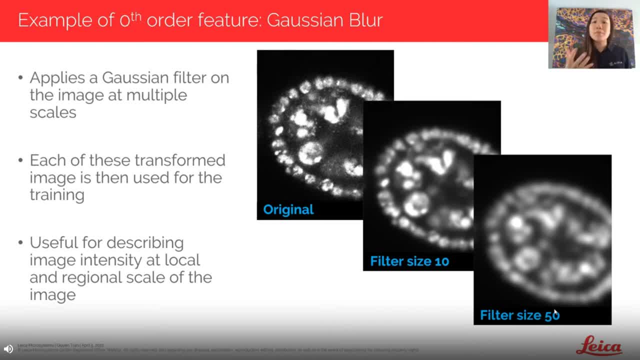 intensity of your objects of interest at a local and regional scale, so that when you're looking at, for example, these large nucleus versus a small nucleus at size filter 10, you have a different intensity profile. then you have at 50, and that might be crucial in classifying these pixels and particularly if you 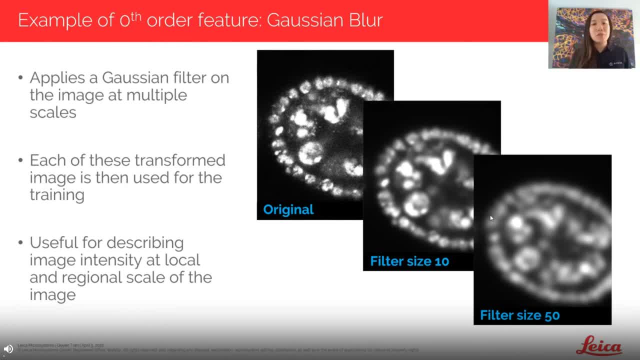 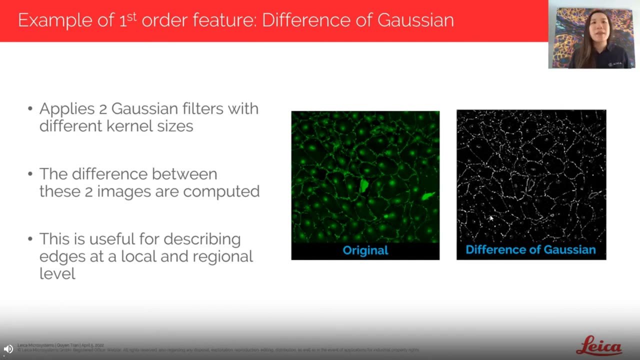 wanted to classify a small nucleus versus a large nucleus. this might be one component that you might want to to. this might be one feature that you might want to use in your, in your training here. my second example for you is a first-order feature, and this is the difference of calcium. what happens here is we apply. 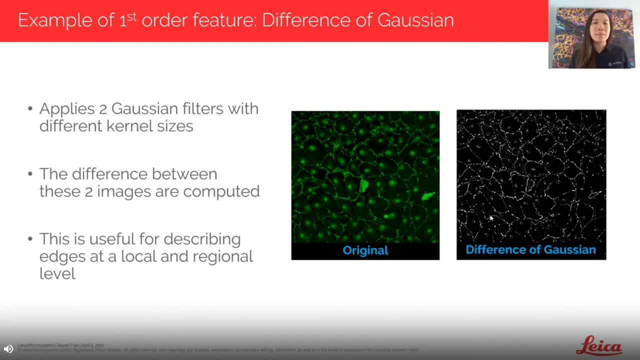 two calcium filters with different sizes and then we compute the difference between those two transform image to get an enough to get another transform image. and this is really good at describing edges, both on the local level and again at the regional level, because we're using different sizes here and you can see from the 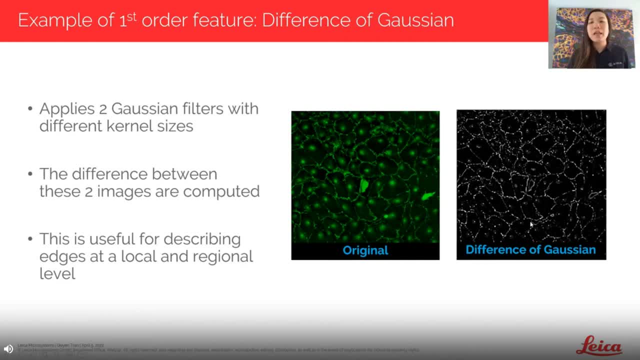 original versus the difference in Gaussian the edges, or particularly the cell membrane in this case, is really highlighted. so this might be a critical feature of calcium that we want to be able to use in classifying these pixels. whenever we're looking at a pixel classifier that is used to amplify or 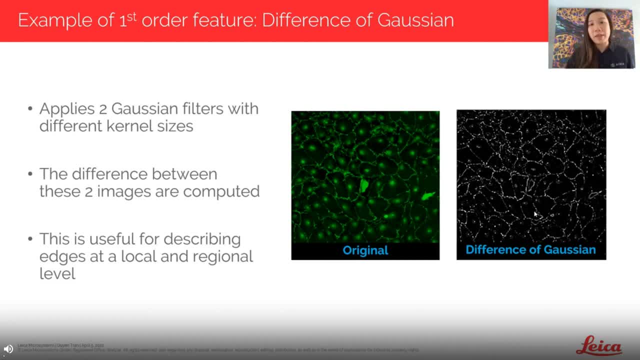 increase the cell membrane and to decrease the signal from the nucleus in this image. so these are some examples of the types of features that are available, and these two are typically used for these these purposes. but again, there's a variety of features that are available here with calcium and calcium, which actually 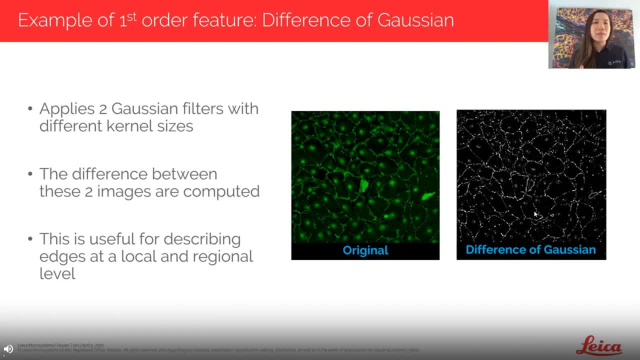 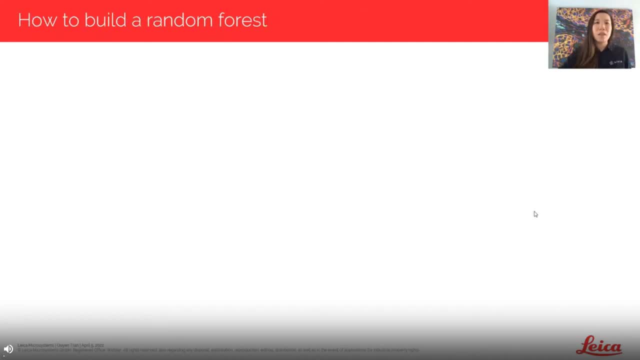 features that you can explore to find the best ones that work for what it is that you're trying to enhance and you're trying to detect. So we've talked about a lot of components. Let's kind of pull it back together and talk about how does this all come together and how do you build this. 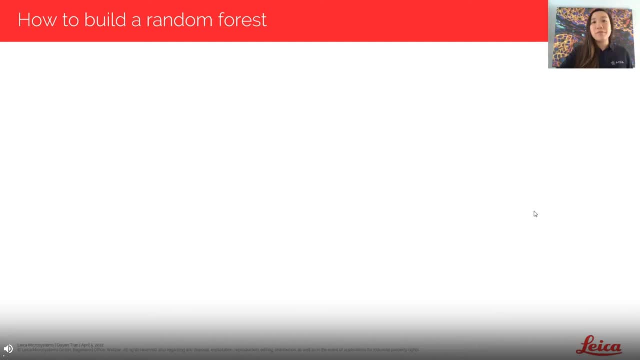 random force, the random force that's critical for your pixel classifier training. So the process kind of looks like this. So we take all of the data with the labels, with our examples, We break it up into random subsets of data. We then teach it a decision tree based on these random subsets. 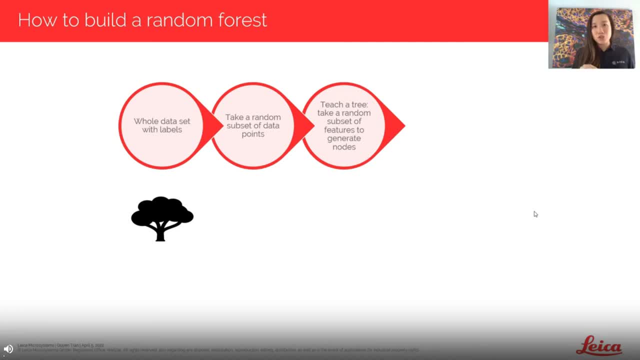 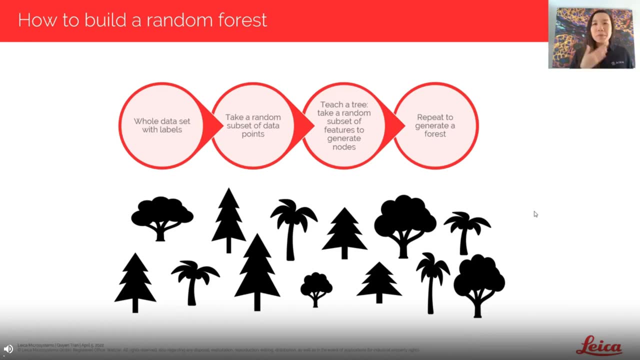 and a random selection of features. So now we have one decision tree. We then repeat this process and because every time we repeat this process we're taking a random subset of the data and a random subset of the feature, each of these decision trees are slightly different. 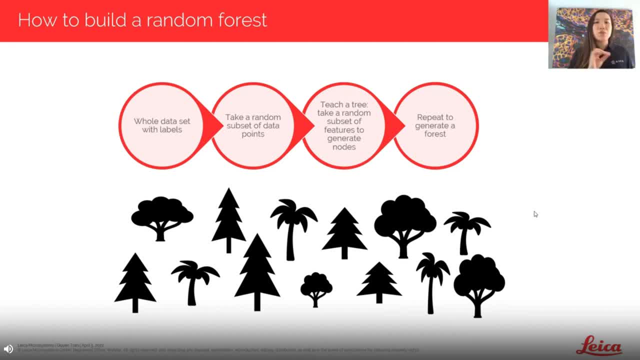 than one another, and what we're trying to accomplish here is all of these trees collectively together make a random forest that is going to give us the best classification of the pixels or the objects into what we wanted versus the background. so you can see from my description. that's kind of where the 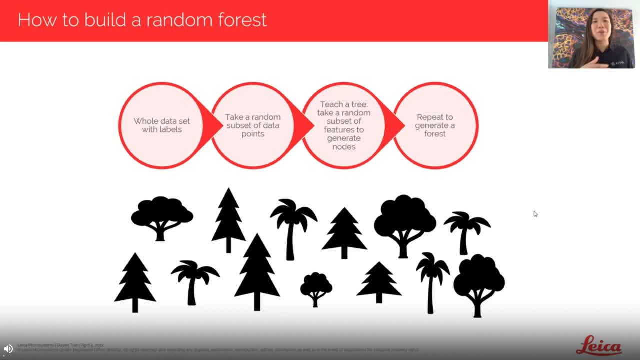 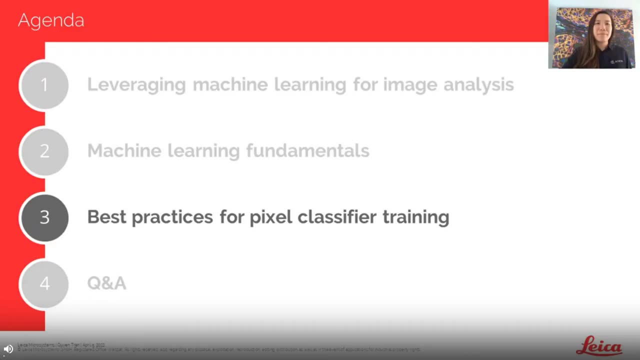 main random forest algorithm comes from right. you're selecting a random subset of things to create a series of trees to pull together to make this classification all right. so let's kind of transition into maybe a more practical approach or a more practical way of looking at this. so now I kind of want to. so now I want. 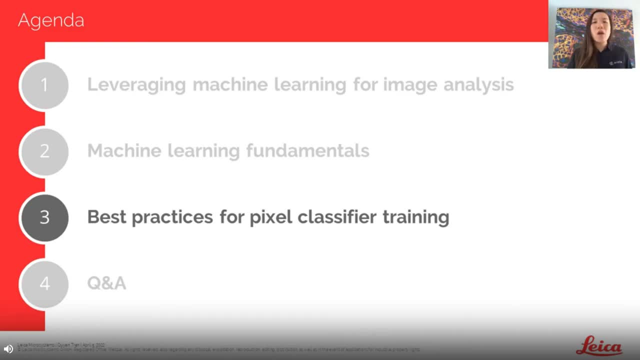 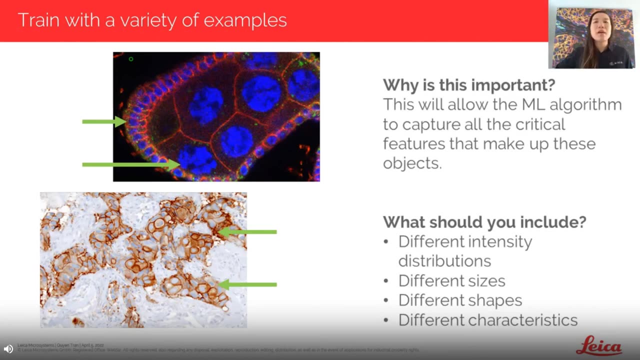 to share with you a little bit more about what we're trying to accomplish here and share with you some of my best practices when it comes to training a good pixel classifier. so my first best practices for you is to train with a variety of examples. now, why is this important? so the machine learning algorithm to make 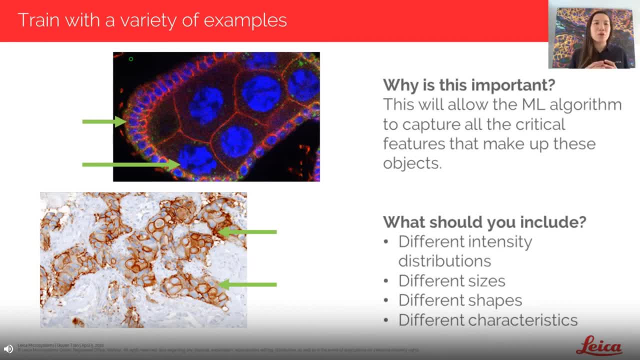 an effective one, we have to be able to capture all of the critical rules, all of the critical aspects of the algorithm. to make an effective one, we have to be able to capture all of the critical rules, all of the critical aspects of the object that you're looking for. so if you don't have a variety of ways that your 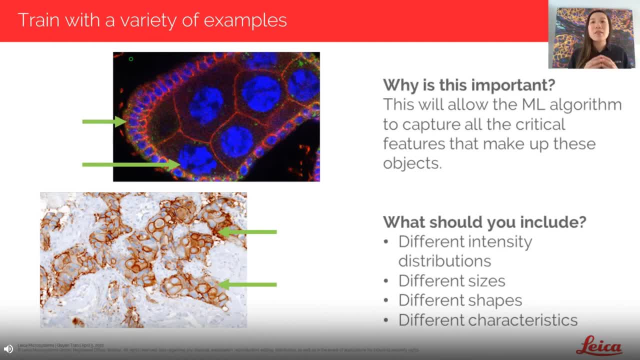 objects can look like, then the pixel classifier in the algorithm is unlikely to pull out the rules that you need. so what kind of things should you include? again, this is not an exhaustive list. this is some that that might be useful for you when you're doing this. so first is intensity distribution. so my 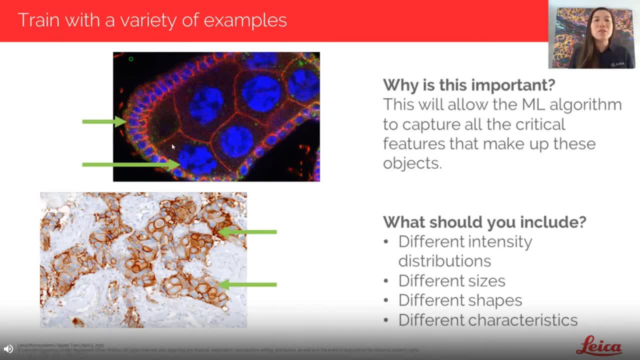 example, with this fluorescent image here, the distribution, we see that was heterogeneous in the large nucleus versus the more homogeneous in the smaller nucleus. you want to be able to capture both of that variation. we're also capturing here the difference in sizes. so if we only taught on the large 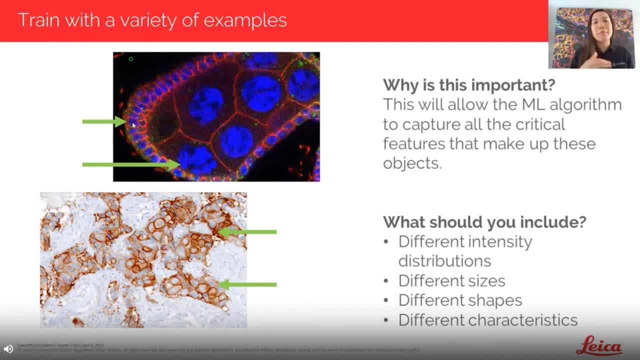 nucleus, we might overlook and might not make the rules necessary to look for the smaller ones too. so you want to you, you want to train and provide examples of that. on both of these. you might also think about shapes and different shapes that your cells and your objects have, and perhaps even other different 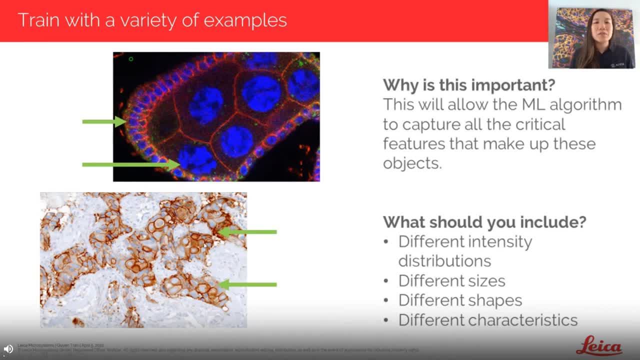 characteristics so down here in the hostology image. what I'm trying to capture here with these arrows is I want to be able to detect areas with some dark staining- so a lot of staining- and areas that have lighter staining, because to me those are still positive staining. so I want to make sure to provide. 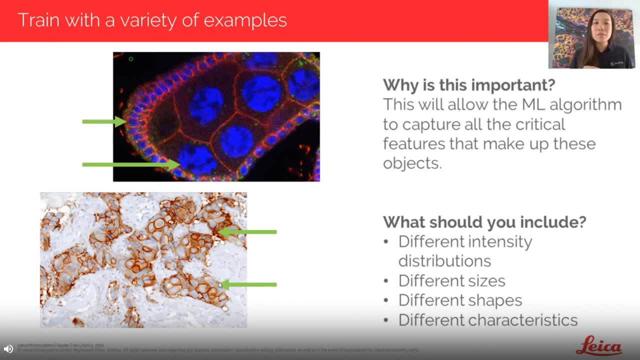 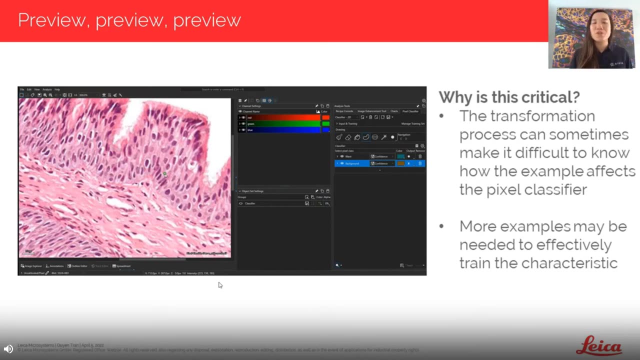 examples of both of those scenarios so that the pixel classifier can learn that those two scenarios are what I want and what's important to me. my other best practice is to preview, preview, preview during the training process, preview frequently and preview a lot in the training process. and why is this? 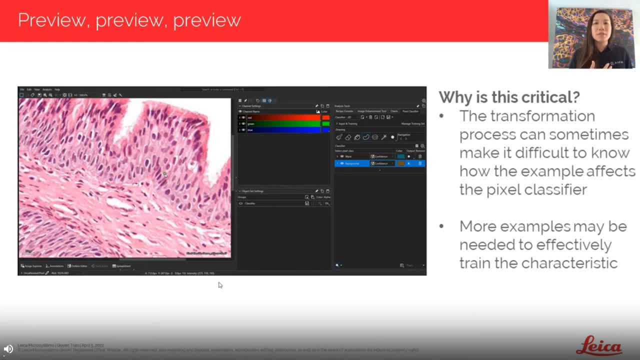 critical for me a lot of times. the the process of transforming the images and the filters into a fully transparent image is very important to me because sometimes, when I'm working with those filters, makes it difficult for me to anticipate exactly how the example is going to affect the final pixel. 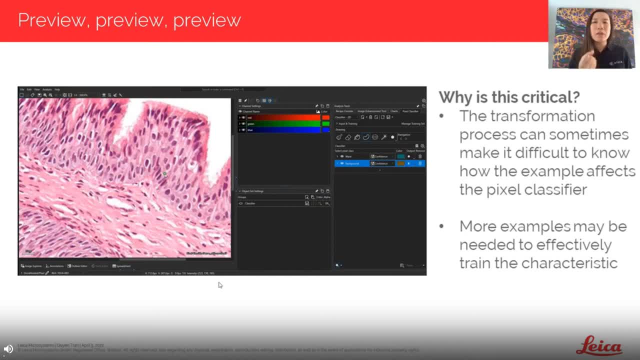 classifier. it's also important because sometimes I find that a feature might be really hard to pull out, those rules exactly. so the pixel classifier might need a couple more examples and it's really hard to know how many examples, what, what's missing and what else to provide. so in this video here i'm starting out with training. 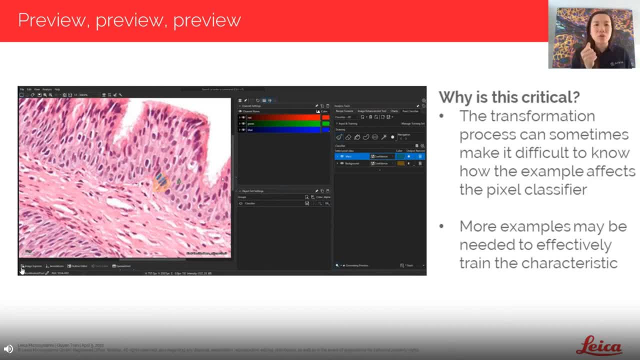 on just these three kind of elongated and dark cells and i'm previewing to see what that looks like. and i find that on my first, first preview i'm not getting these round nucleus here. so now i'm going to teach it on that, this last round. i'm finding that while i'm getting the round nucleus 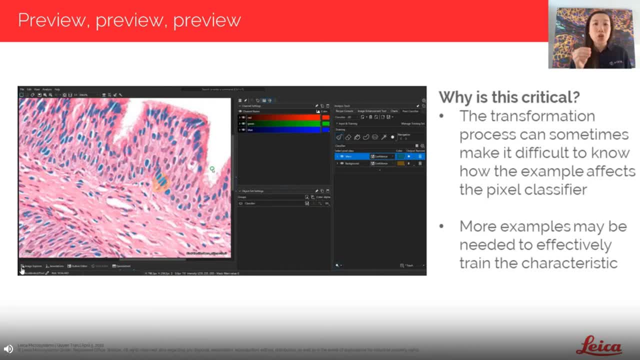 i'm not getting the ones that are not super dark and super well stained. so now i'm including that. so basically, during this previewing process, it gives me an idea of what's missing. what else do i need to provide to the pixel classifier to make the best one possible? so by previewing not, i'm not. 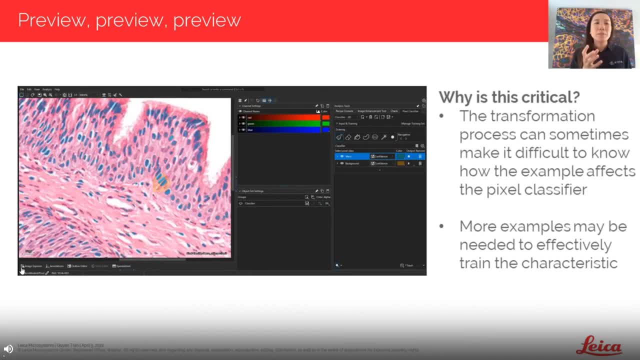 only seeing what is being detected, but i'm seeing where things are missing, so i can add just that component. it's going to save you time and it's going to basically allow you to kind of just look at the results and not think about this entire transformation process and how things will affect the pixel classifier. 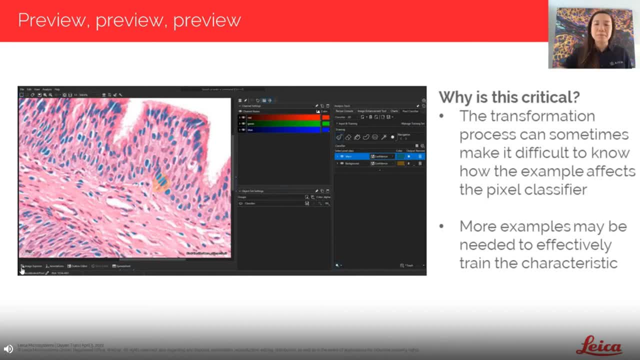 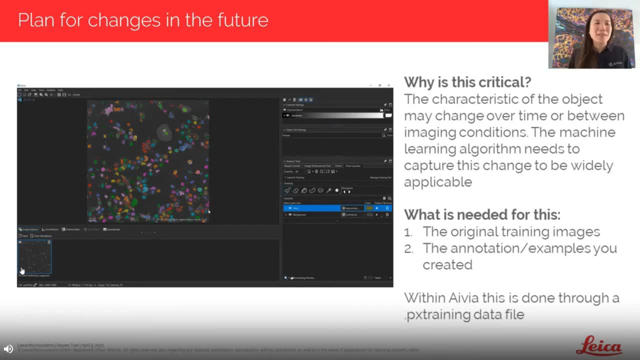 based on this transformation process, and my best third practice for you is plan for changes in the future. um, i know, as scientists we we typically encounter changes a lot. our experimental conditions change or our imaging parameters change. you can never really plan for everything. things happen, and so i like to kind of in my pixel classifier training plan for the fact that things are going. 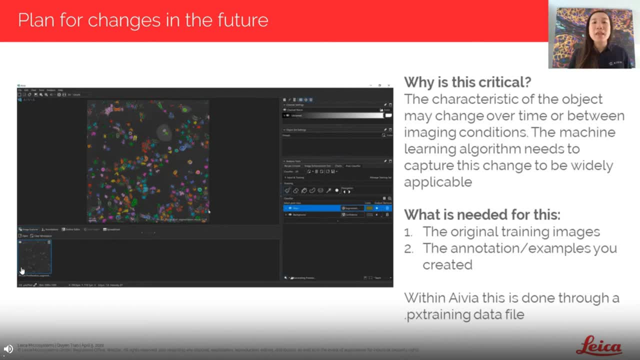 to change um. so what happens in avia, it's particularly is: avia allows you to save what we call the pix train data file. what that includes is a pointer to your original data and then all of the examples you provided. so when you pull this PIX training data out, you have these two critical components to train the PIX. 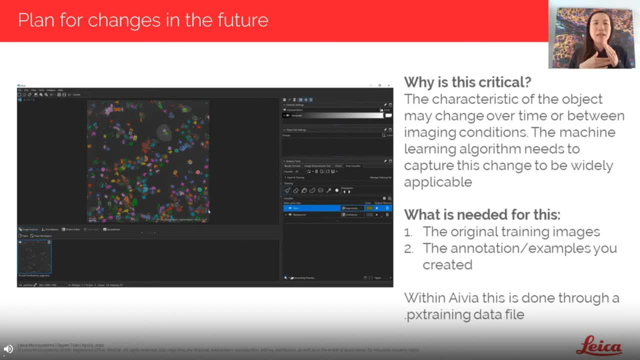 classifier again And it allows you to add in more data, more examples, to make the PIX classifier that you really need. So in my video example here, I started out training on a image that has a low cell confluency. I apply it to one that has a higher cell confluency and realize 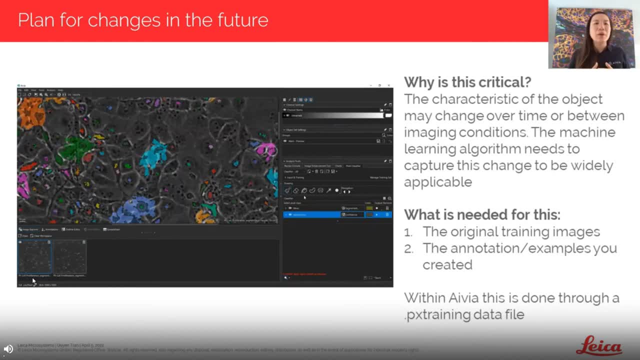 this isn't great. It's not picking up what I wanted to. So now I'm going to actually go in and add more training, add more examples, particularly from that higher confluency image. So with something like the PIX training data file, I can do that And I don't have to necessarily. 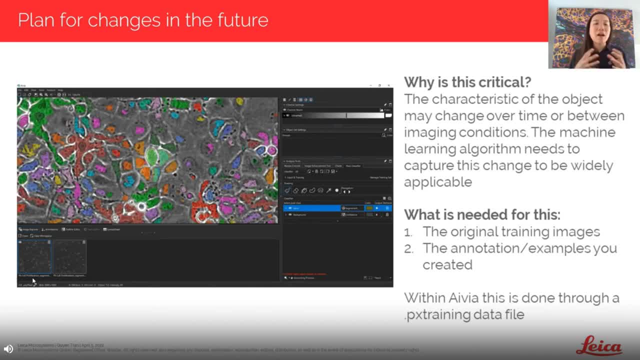 plan and have the data up front. when I'm training the original file, I always have the ability to go in and make the training data. So I'm going to go in and make the training data And I'm going to go in and make the training data. And I'm going to go in and make the training data And I'm going to. 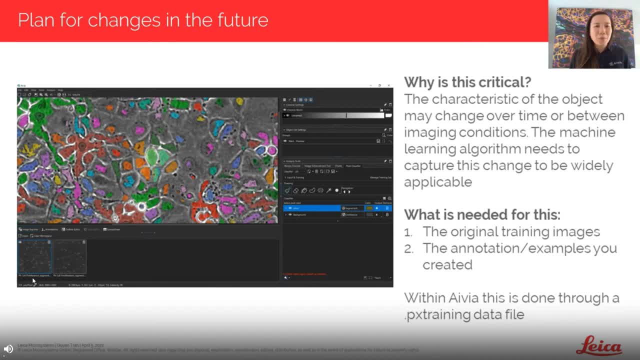 modify it later. So I always tell people whether you think this is the best PIX classifier you've created and the one that you're always going to use. it's a good idea to basically have this PIX training data file, just in case something happened. Just plan for things that change Plan. 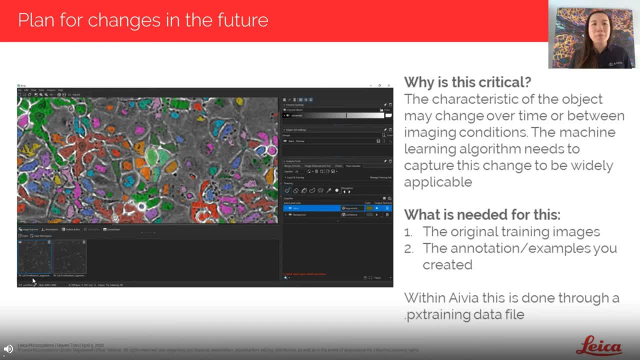 for the future. Give yourself a little bit of a break, because sometimes going back and training it from scratch is difficult, Depending on how long and how difficult it is to create the PIX classifier training in the first place. So those are kind of my three best practices for you. Train with a variety of examples. Preview: 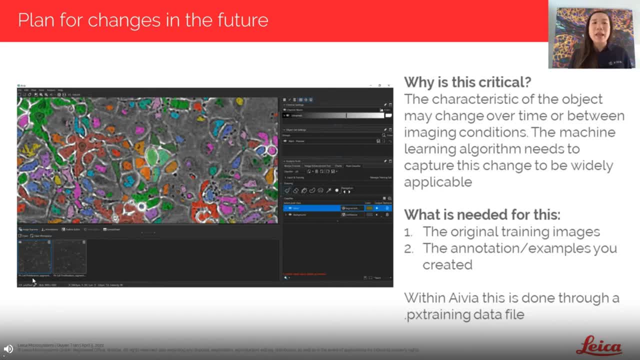 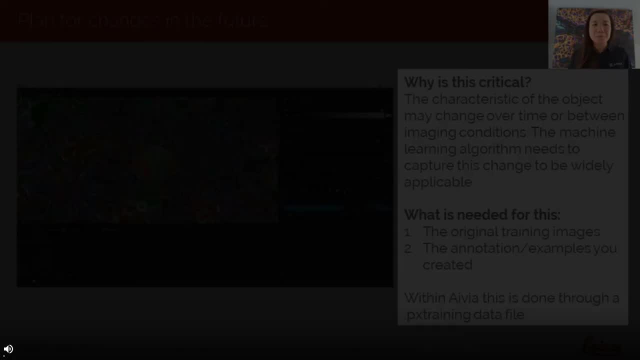 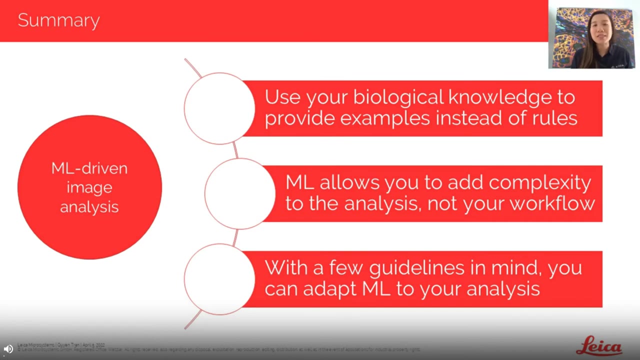 constantly when you're changing, when you're training, And always have a plan for the future, when things may or may not, when things may change for you. All right With that, I would like to quickly summarize The presentation that you've seen today. I hope in this webinar you've seen that machine learning. 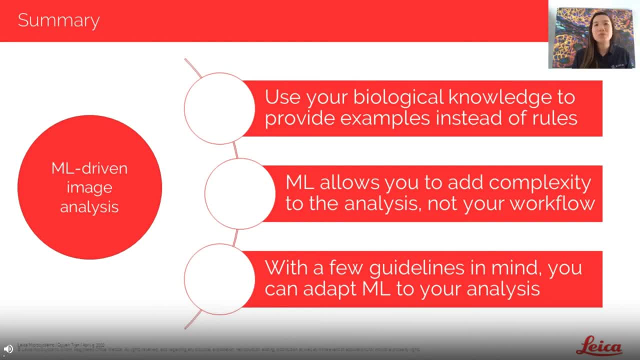 driven image analysis really allows you to leverage your biological knowledge in providing the examples to the PIX classifier instead of the rules, And by doing it this way, we have the capacity to add complexity to the analysis, because the PIX classifier can provide you rules that you 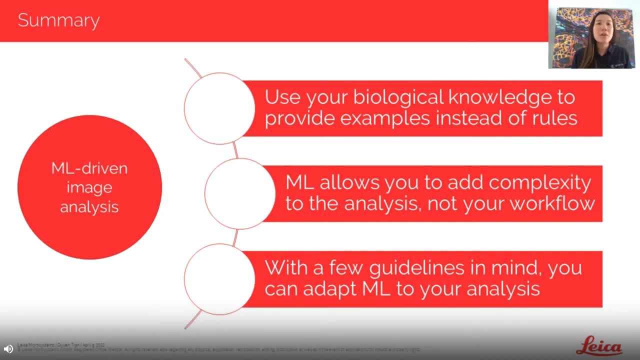 may not have considered Or may not have thought about, But this complexity that you're adding to the analysis doesn't necessarily have to mean that you're adding complexity to your work. The painting of examples make this fairly straightforward and a really easy way to basically do the image analysis. I also hope that you've 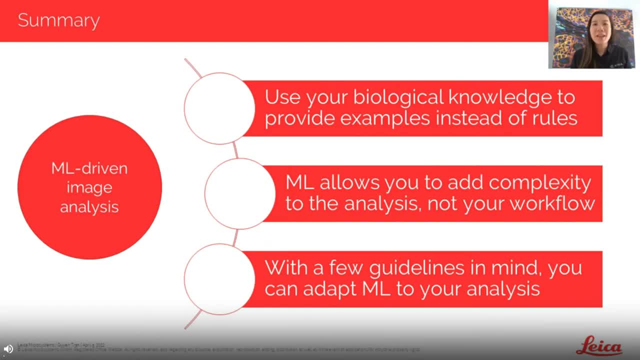 gathered some useful tips and a few guidelines to keep in mind When you're doing machine learning- pixel classification training- and that these guidelines really help you to create a classifier that's very effective and really useful for what it is that you're trying to detect and trying to do in your research. 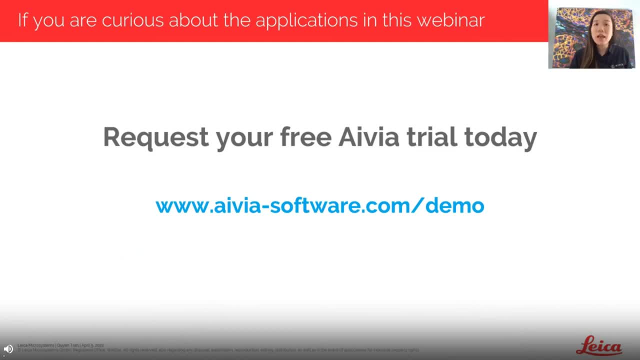 I also want to let you know that Avia does have free trials. So if you've been curious or you want to try out the pixel classifier or any of the examples I've shown you, such as going from a phase contrast image to segmentation, that's available in Avia. 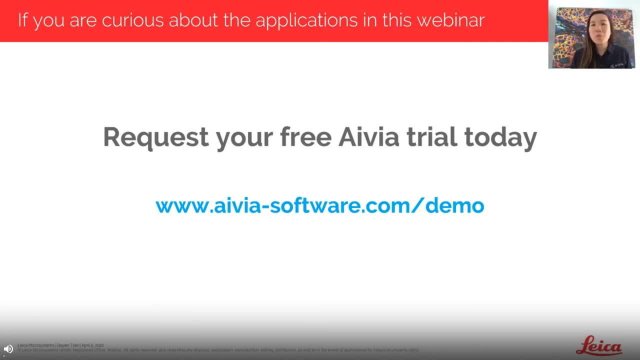 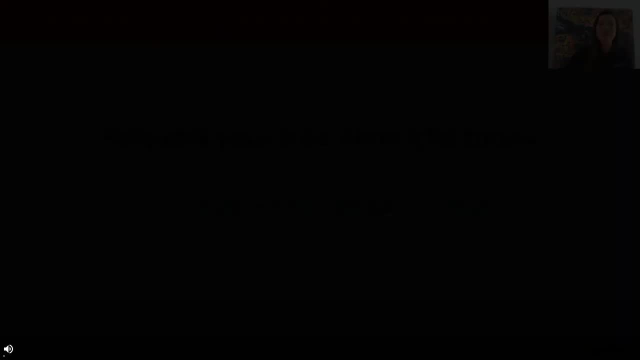 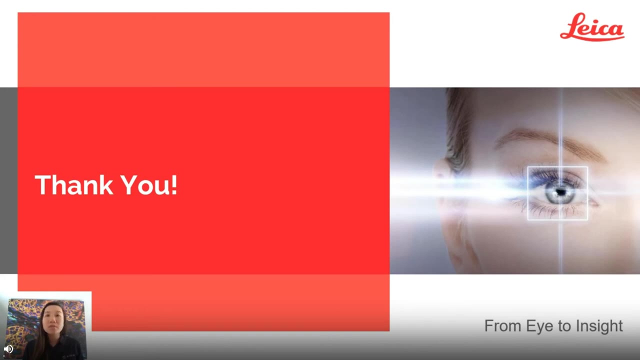 You can give it a try for free today. Just go on our website avia-softwarecom slash demo to request your own free trial today. And with that I want to say thank you again very much for attending this webinar. I hope you found it useful And now I'll be happy to take questions that you have regarding the PIX classifier. 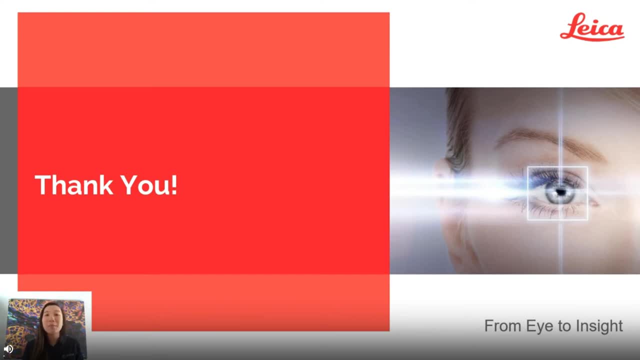 The information I presented today. I'm also going to go ahead and invite some of my colleagues to join me in this Q&A session, just to provide me with a little bit support and resource so that we can make sure that all of your questions are answered. 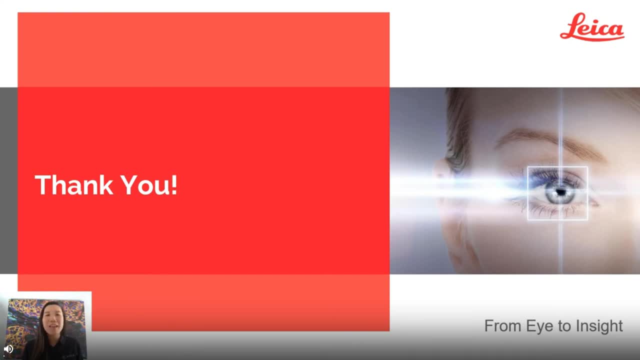 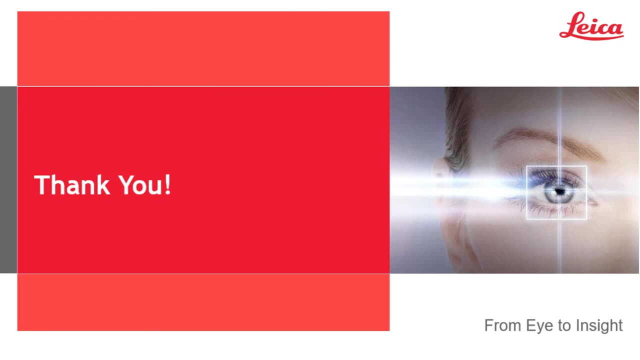 Again, thank you very much for attending today, And now I'm happy to take any questions that you have. Thank you, Dr Tran, for your informative presentation. We would again like to thank you for joining us today. Thank you, Dr Tran, for your informative presentation. We would again like to thank you for joining us today. 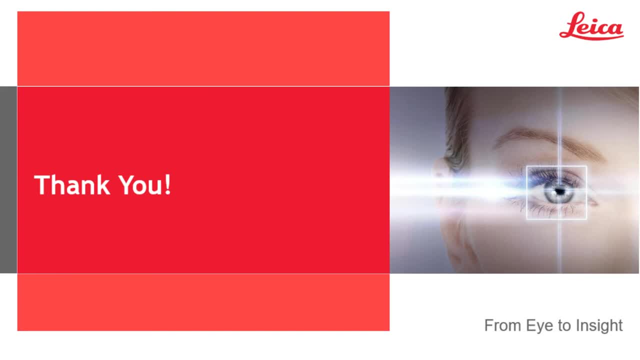 We would again like to welcome Hoyin Lai as we begin the live Q&A portion of the webinar. If you have a question you'd like to ask, please do so now. Just click on the Ask a Question box located on the far left of your screen. 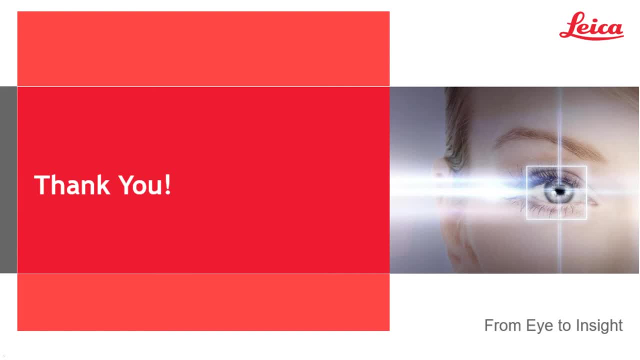 We'll answer as many of your questions as we have time for, So let's get started. Our first question is: does machine learning require a powerful computer? Yes, So for machine learning you do not need a very powerful computer to run the pixel classifier. 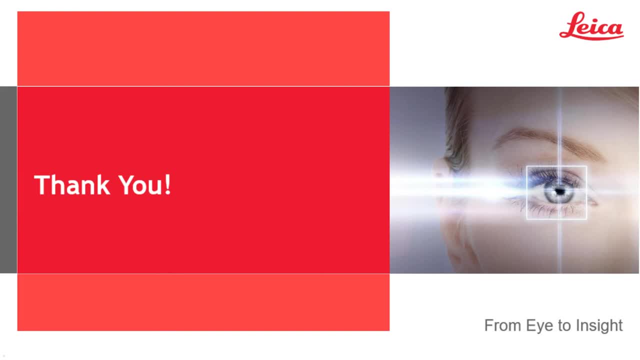 Essentially, what we have implemented in Asia is that it will default to CPU processing when a GPU power is not available, Or let's say, certain features actually do not have GPU acceleration, and that will also default into using the CPU as well. Of course, the performance will be a little bit slower compared to 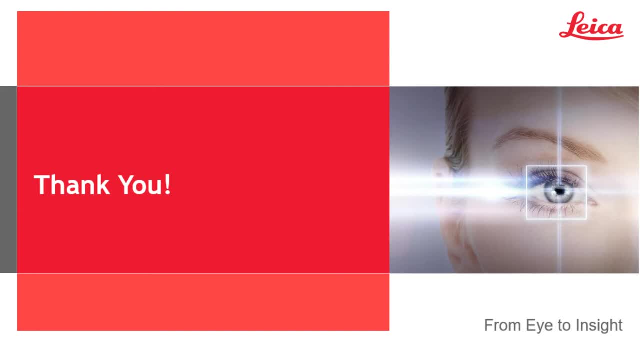 using a GPU, but otherwise you do not need to have a very powerful machine to use the pixel classifier. thank you. next question: once I've trained a pixel classifier, can I apply it to multiple images? yeah, so with the pixel classifier you can apply this to multiple different images. what you have. 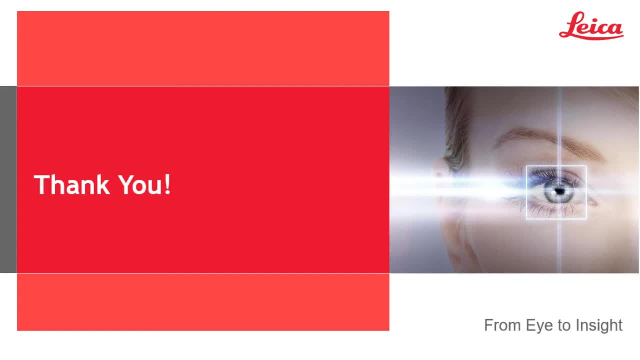 actually trained on. with the pixel classifier, it's not specifically the information that is that is on that image that you, that you have, but rather the other information that is encoded. so that allows you to, as long as your experiment or your imaging condition doesn't change too much, you will be able to apply the pixel classifier to other images in your experiment. 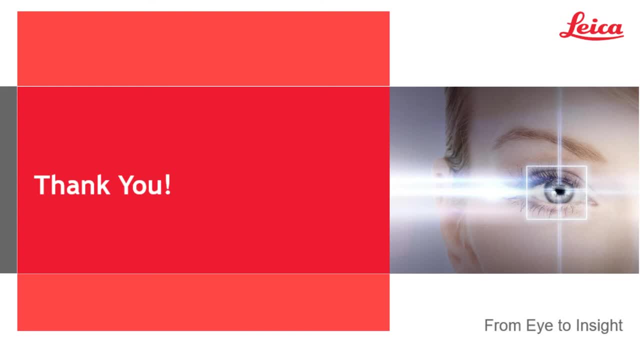 and, of course, if you do, once you, when you apply the pixel classifier and you realize that it wasn't performing as well as expected, you can also add those images to your training data set so over time you can build a much more robust pixel classifier for your application. thank you, next question: 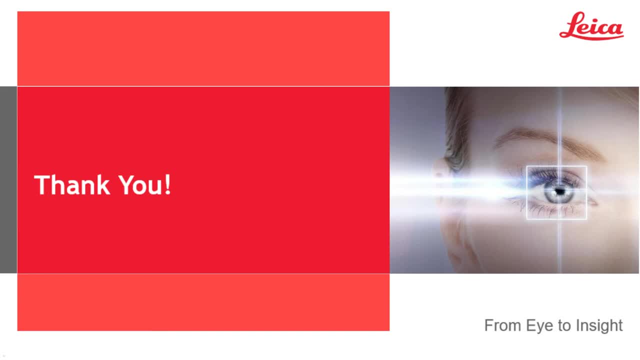 it is possible to use the ml tools in my? is it possible to use the ml tools in microscopy images of mammalian fish, amphibian oocytes or eggs? I wonder if development of different stages could be analyzed and recognized. what kind of image processing tools do we need to analyze that? 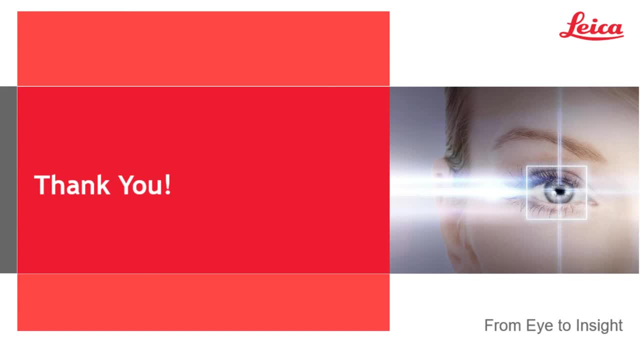 kind of those kinds of images. so I'm going to assume that in this case, we're looking at the development in the early, in the early development cycle. so in that case, yes, it is going to be possible to use the pixel classifier to analyze these images, and the one thing that we actually 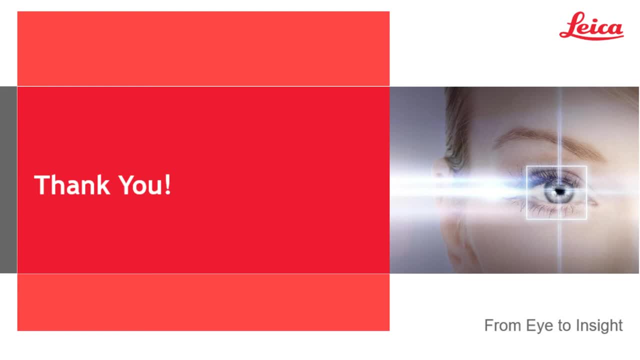 uh, with the pixel classifier, is that? um? for, for instance, if you were looking at the different thermal layer organization, you just need to paint kind of the specific regions that you're interested in and, um, the pixel classifier will try to kind of identify those and for um those, 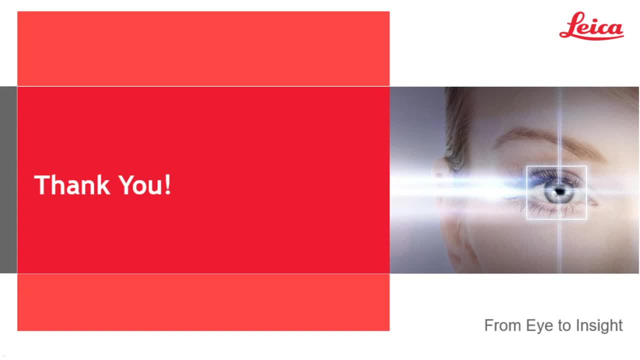 regions, based on the information that you provided. so perhaps, maybe, for example, maybe in some cases- that the nuclei are maybe a little bit smaller or there is a visible cleft in the data on the image, so some of those things could also be picked up by the pixel classifier as well. 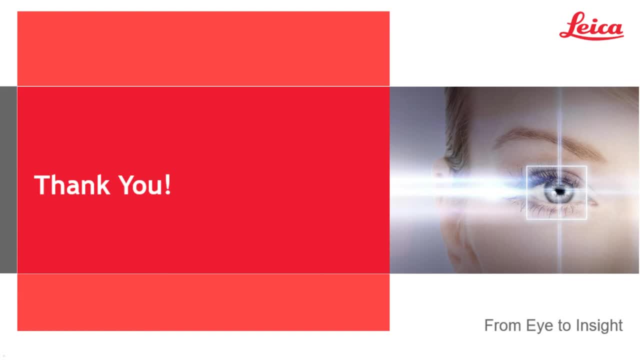 great, thank you. next question: how do people document and share their pixel classification protocols? uh, so, um, yeah, so, typically the pixel classifier, um, the um, the file will be saved, you will be saved to a specific file and that you can take that and you can apply it or to other um. you can load it in another copy of asia that your colleague has or if you. 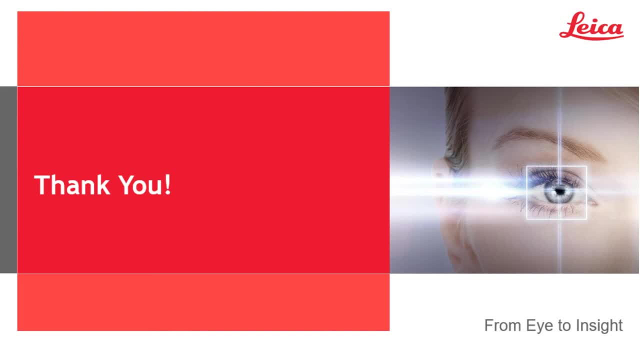 are just trying to train a pixel classifier. you can use asia community, which is our version of the freeway which allows you to load and train a full copy of asia to apply and also like in terms of documentation. sorry, sorry, um, for documentation. um, the information about which feature gets used- uh is available and the pixel. 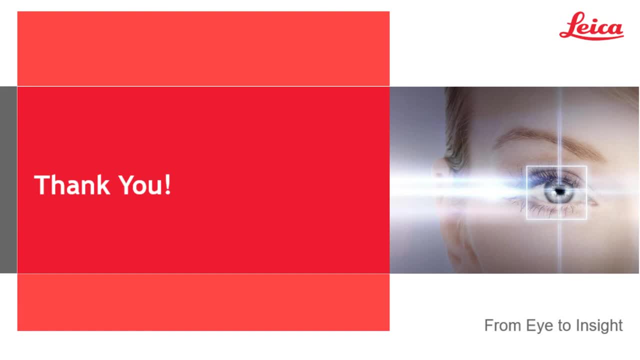 classifier as well. so when you select uh, when you train a pixel classifier, you can select which feature that it will um that you want to apply uh, apply with and that, and, and. you can have that record as well. great, thank you um next question. hi quinn, thanks for the great talk. how does the 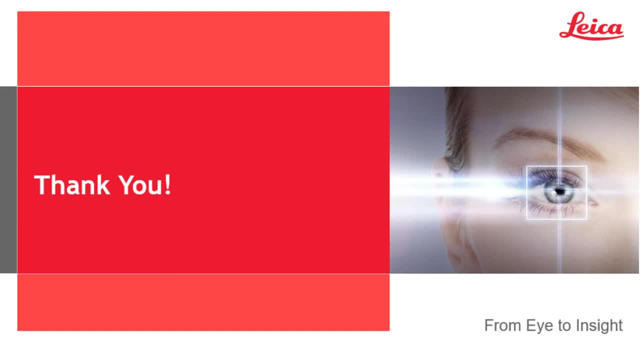 perform? how is the performance of the pixel classifier available for the pixel classifier an avia? um, thank you very much, uh for for that comment and for the performance. i'm assuming, um, we're talking about the, the, how well the pixel classifier detects the signal, or the Sixto Classifier. 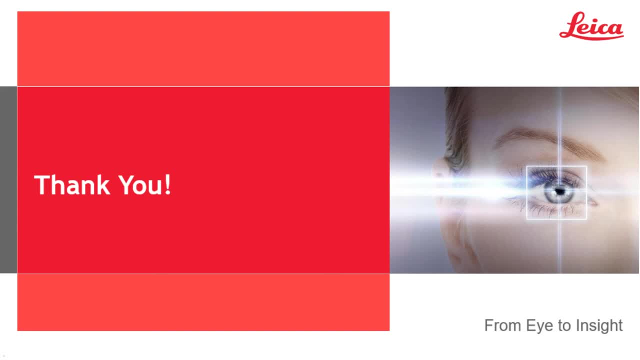 object of interest that you want and that's really based on your review of the results, so kind of like the pixel classifier. so, out of all the results that you can expect possible in the cortisol performance, but it's also um also possible, such as the Institute of Machine Style component. in the case that the pixel classifier vegetables and editing the screen, pas chama, the particle basicallyass harbor. that shows the levels in which you want to collect the particles by the pixel classifier. the first sheet of the slide shows all of the observation that we have to do to場as the task intéress a. 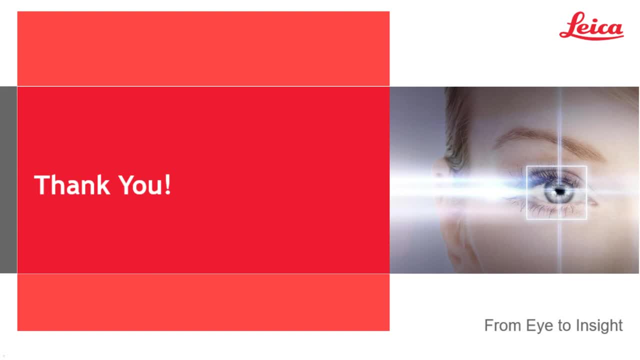 preview or we can also look at the final results. You, as the expert, is the person who will assess how well that pixel classifier looks and how well it performs. So once it's applied, you can straightaway look at what cells are detected and whether or not that. 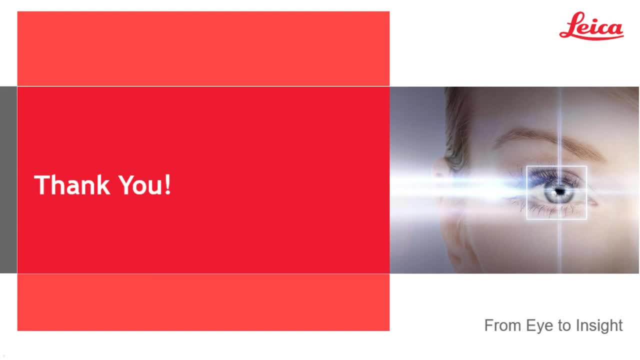 fits your criteria for a good performance or not? Great thank you. Next question: what is the minimum size of labeled data set that gives good performance? Ah, yes, we get this question asked a lot and unfortunately it's not one I can give. 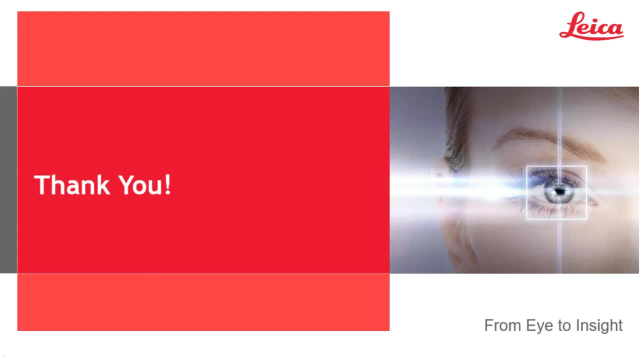 you a answer on. basically, It varies quite a bit by what it is that you're trying to enhance or you're trying to improve. It varies by what it is that you're trying to segment. As we saw in the example of the training process, it can be just a small region of interest. I have done this with just an. 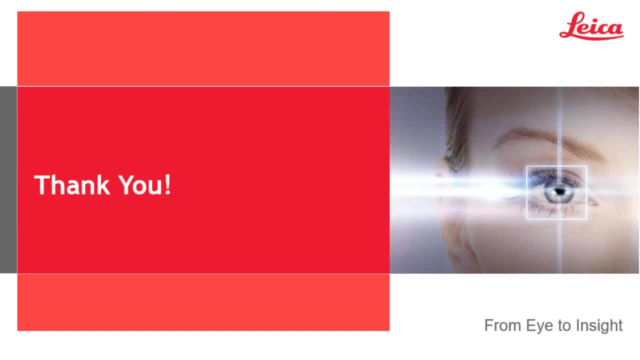 example of a few cells and I've done this where we've had to do a couple of previews and 10, maybe 15 examples and things like that, Great things like that. so it varies quite a bit, but that's one of the reasons why that preview. 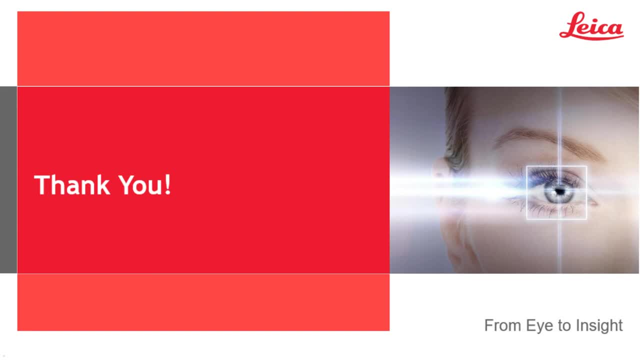 functionality is immensely helpful because you can look at it along the way and see how well it's performing and add just enough of what is needed to get a good pixel classifier. so, again, it really varies depending on what kind of image analysis you're looking for and the images that you're 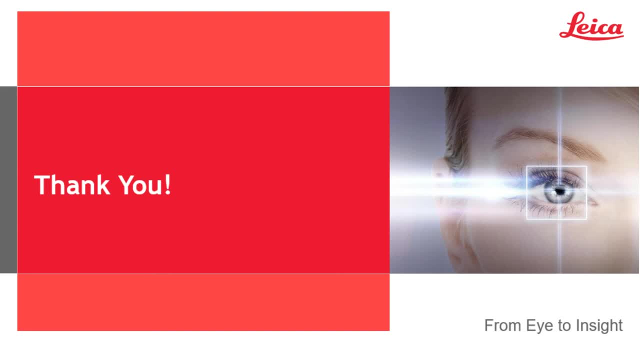 kind of starting out with all right, great, um. next question: how well does avia play with other image analysis programs such as fiji and file formats? so, um, i'll take the file formats first. uh, so for file formats, avia can read a number of file formats. i can't remember the exact. 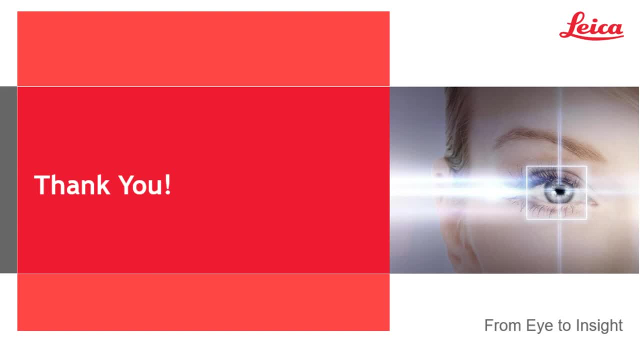 amount of the top of my head, but at least 15 kind of file formats natively. so that's just us reading directly for file formats that we don't cover. we do have a bridge with bioformat a, a script or or kind of an application in fiji that covers. i think they're up to. 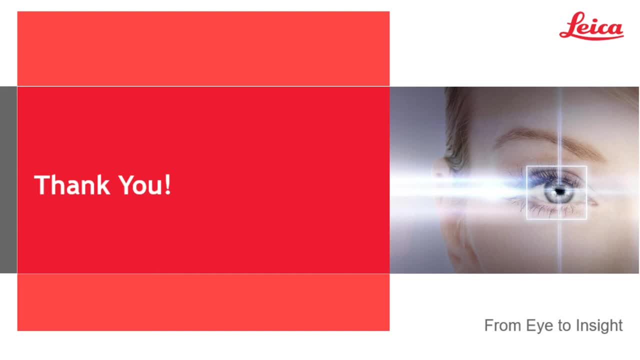 like 400, maybe 500 bio formats now. so there is that bridge if we don't cover the file formats that you need in terms of kind of how well it works with other programs. so avs optimize for tips, which other programs that there's- fiji and in general other image analysis analysis program.